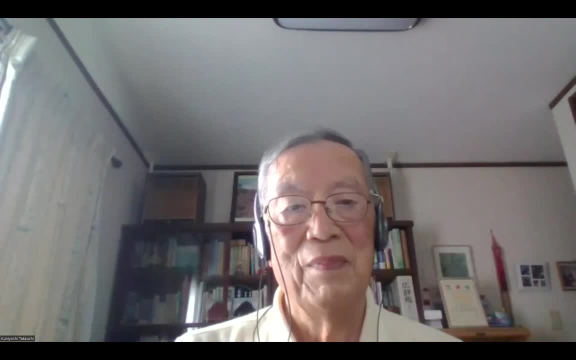 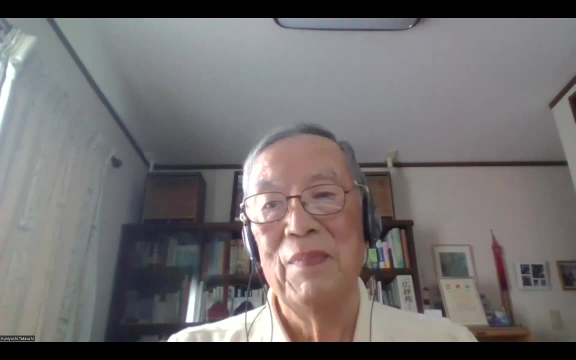 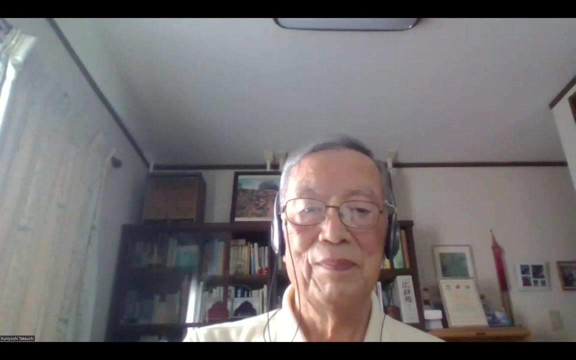 Takeuchi is a Professor Emeritus of University of Yamanashi, close to Japan, where he taught hydrology and water resources for 30 years till 2007.. And and I'm also fortunate that I was his student student during his his professorship in University of Yamanashi. so 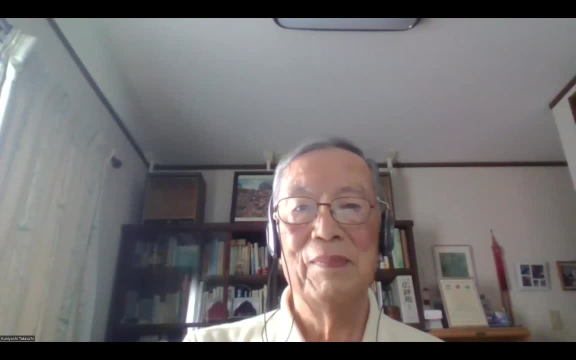 I still recall, you know, many good experiences and and a lot of activities in university of yamanashi. he served as the founding director, and later an advisor, of international center for water hazard and risk management, which is popularly known as icham. under the auspicious of unesco chukuba, japan, he got his bachelor of 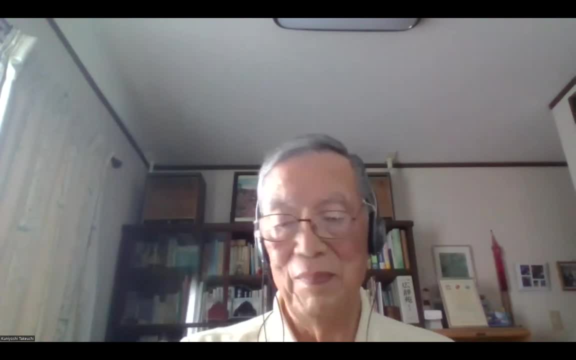 science and master of science, and later um doctor of engineering in civil engineering at university of tokyo and phd in city and regional planning at university of north carolina in the usa. he has been specialized in surface hydrology, water resources systems and disaster management. 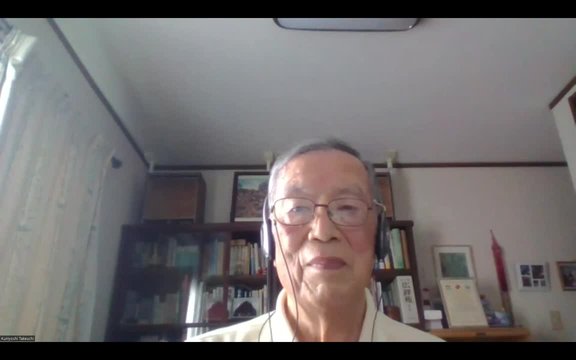 he served for various professional offices, including the chairperson of intergovernmental council of unesco, isp for national. the president of ihs for 2001 to 2005 and the chair of iugg commission of geophysical risk and sustainability for 2007 to 2015. a vice chair of scientific committee of 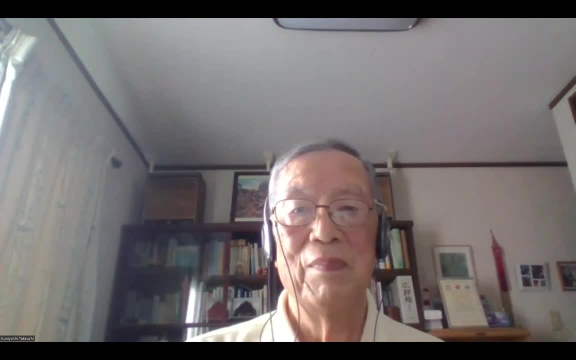 issu, issc, unisdr- integrated research on disaster risk for 2009 to 2015.. he's a recipient of several professional awards, including ihs, unesco, wmo, international hydrology prize in 2012.. so, with this brief introduction, i would like to invite professor takeuchi to 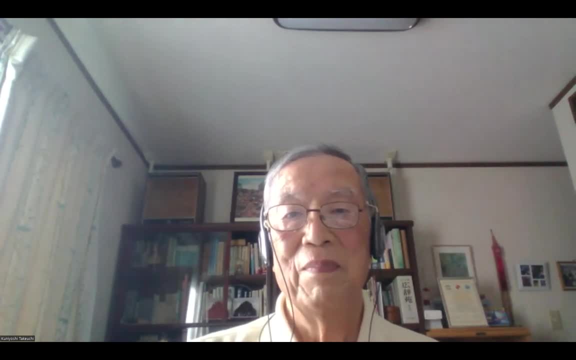 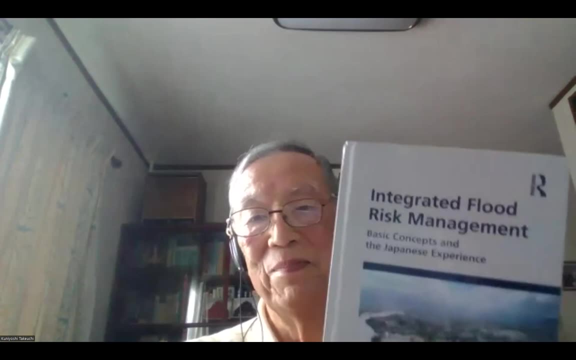 introduce his book on integrated flood risk management: basic concepts and japanese experience. and also i would like to inform you that we have at least 30 students inside the university of unesco, university of west korea, and also at the university of india, our classroom here at AIT. 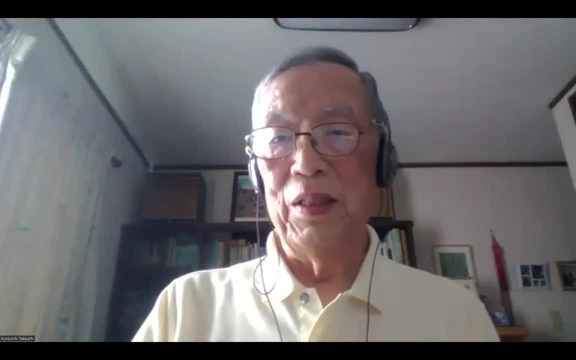 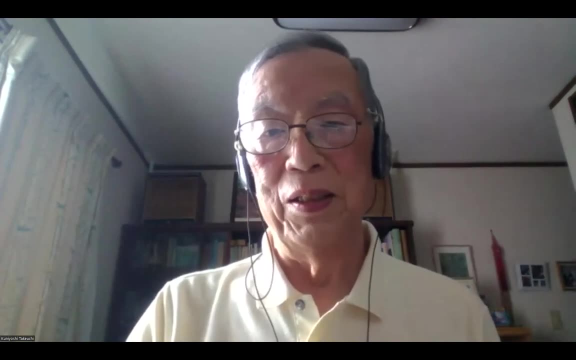 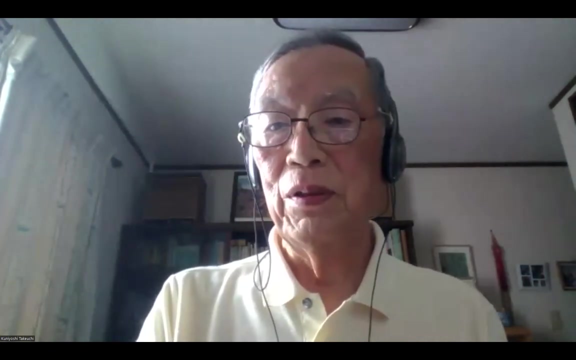 Thank you, Professor Takeuchi. yeah, Okay, thank you very much, Sangam. This is really my honor to speak to the people at AIT and other places. Well, I went to AIT for the first time 1975.. 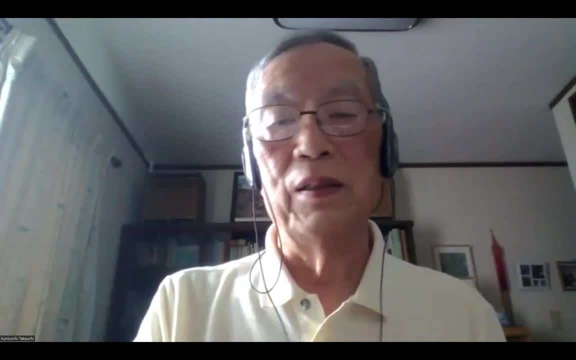 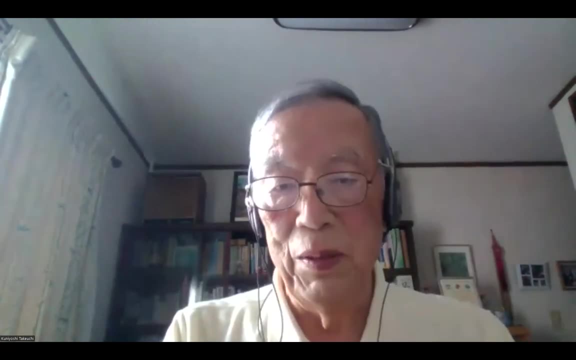 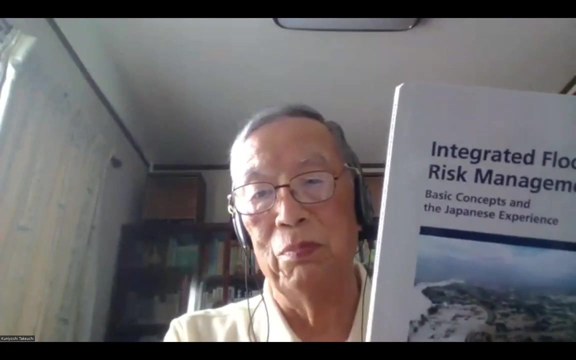 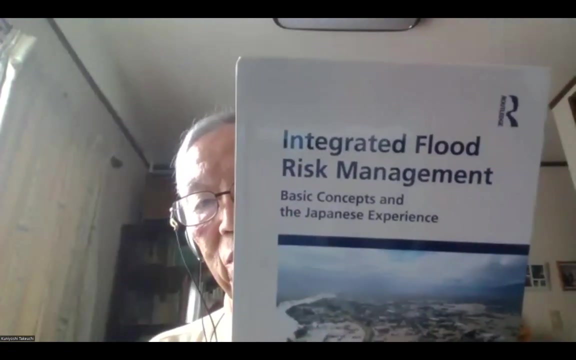 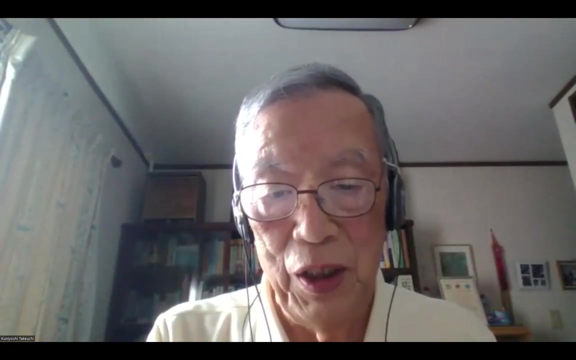 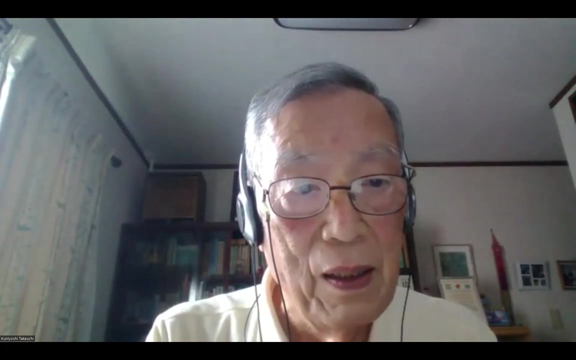 1975,. many of the students haven't maybe been born yet. Today, I'm very happy to introduce my book about the integrated flood risk management, And I hope I can explain this well. Well, I'd like to share the Yeah, yeah, yeah. 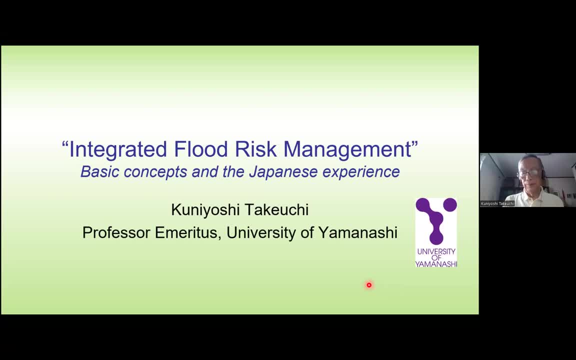 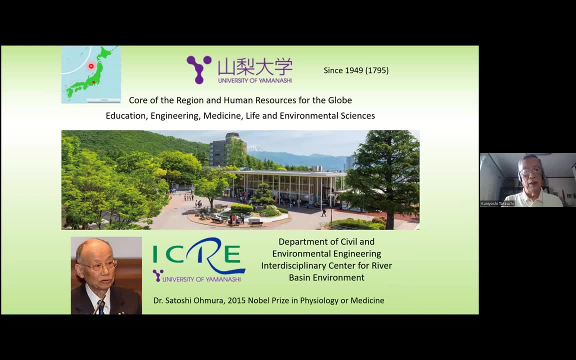 Before starting this, I'd like to introduce my university, Yamanashi. Yamanashi is located in the center of Japan, and this is since 1949. and well, I think- And we have among our graduates- there is a Nobel Prize winner also. 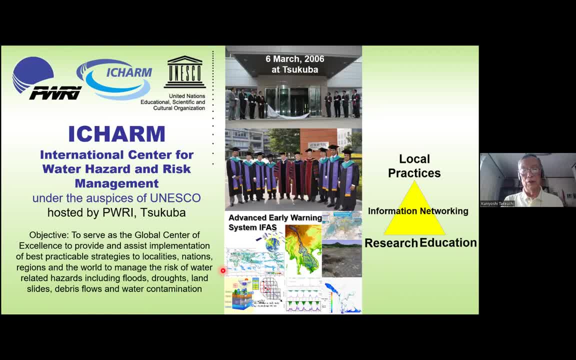 And also I was, as Sangam introduced me, I was at ICHAM after my retirement of at the University of Yamanashi, And this was the under the auspices of UNESCO hosted by PWRI and Tsukuba. 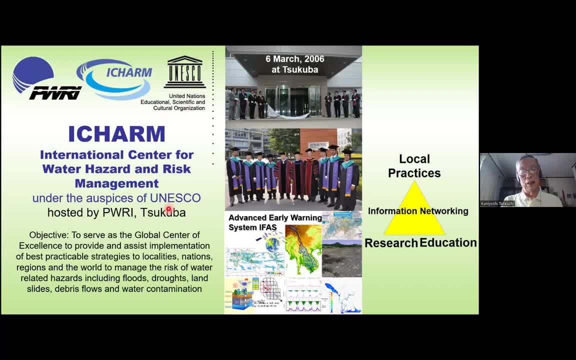 Well, this is the institute working for or together for UNESCO, And we have the education program and the research program, And the research and the education are two fields of our vehicle and the information networking is our navigation And our the ICHAM car vehicle is towards local practices. 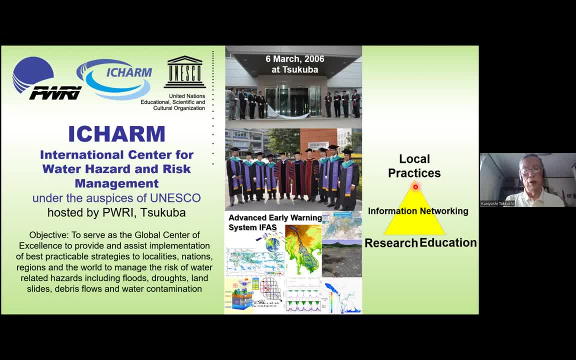 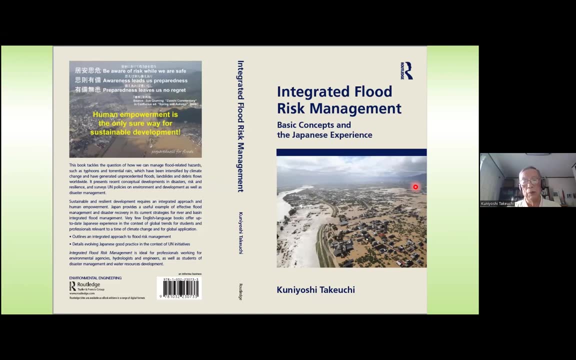 And we do help the local people to do that, And we also offer a special training on the Visual Railway for various kinds of transportation on the platform, And I think that's all I have to say Thank you. Thank you for having me, Mr Yamashiro. 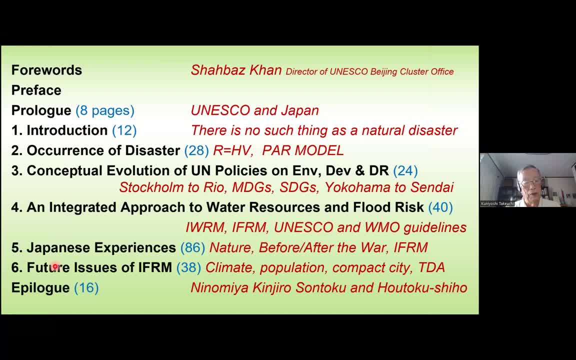 And thank you, Mr Yamashiro, for having me. Thank you, Mr Yamashiro, for having me. This book has six chapters, six chapters starting from well forwards, by Shabazz Khan, who is the director of UNESCO Beijing Cluster Office. 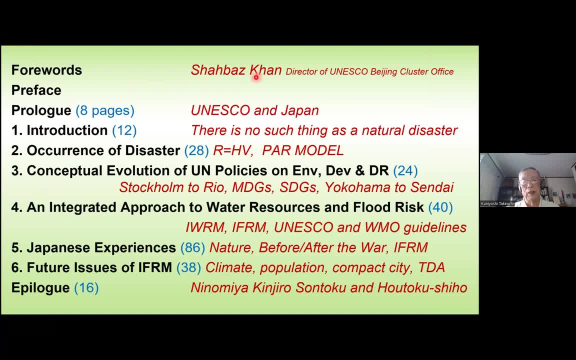 because I'm engaged in UNESCO matters quite much. that is why we have his forwards And also I-CHAM is under UNESCO And preface and the prologue and I have an epilogue too, And the prologue is about UNESCO and Japan. 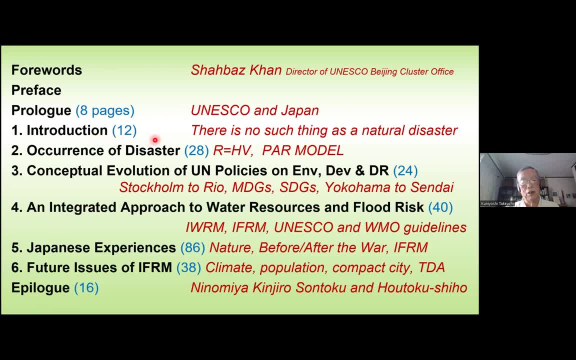 and the chapter one introduction highlights there is no such thing as a natural disaster And the chapter two occurrence of disaster. that highlight risk, disaster. risk is combination of hazard and vulnerability. This is very important And the so-called pressure and the release model. 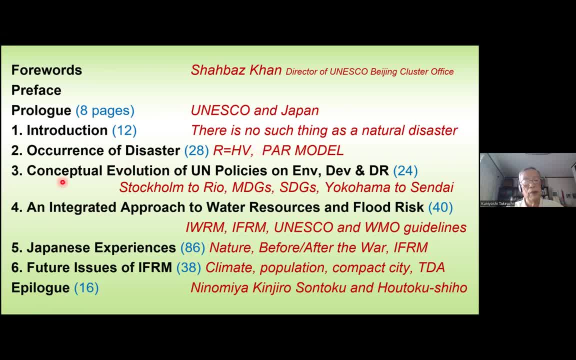 power model is introduced. Then chapter three, about the conceptual evolution of UN policies on environmental development and disaster reduction. And this is really important because the world is now quite much led by, you know, by the international trend And the UN policies are quite important. 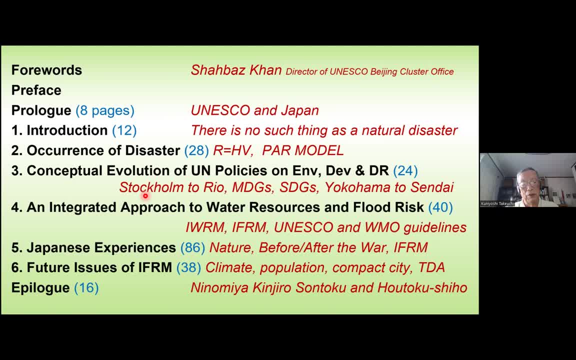 And I work for I will present Stockholm to Rio and Yokohama to Sendai. Then the chapter four is the integrated approach to water resources and flood risk, where I introduce the, the international views or international understanding of those concepts, And then Japanese experience, as you see. 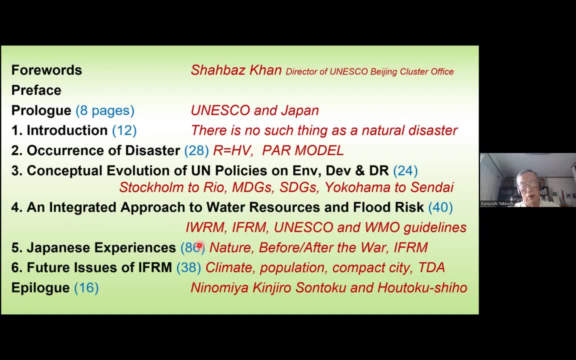 this is a number of pages, So this is a very big pages. about a half of this book is about the Japanese experiences And this is a start- from nature and the history and the current integrated flood risk management And the future issues. I touch upon climate and the population. 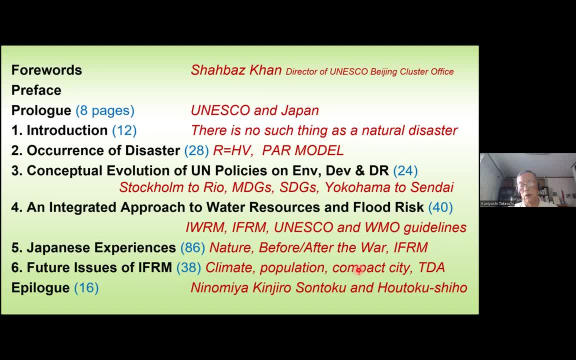 And as a solution, I talk about compact city and transdisciplinary approach. And finally, in epilogue, I introduce Nino Miyakinjiro Sontoku and his policy Hotoku Shihō, which is he was the disaster management saint. 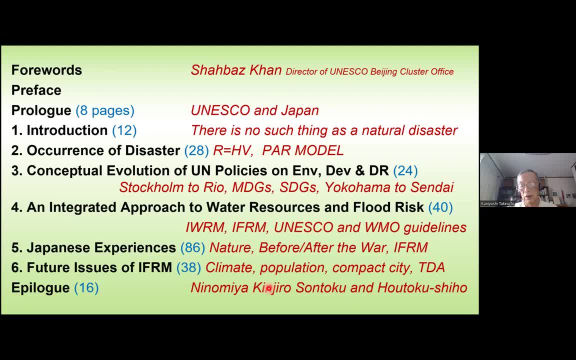 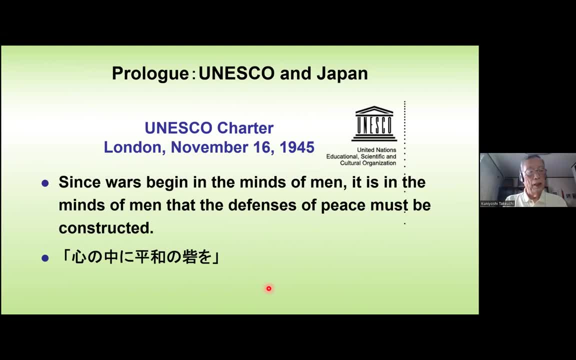 well, disaster recovery saint in Japan. Well, prologue, the reason why I got engaged in UNESCO was because of this charter, Since wars begins in the minds of men. it is in the minds of men that the defenses of peace must be constructed. 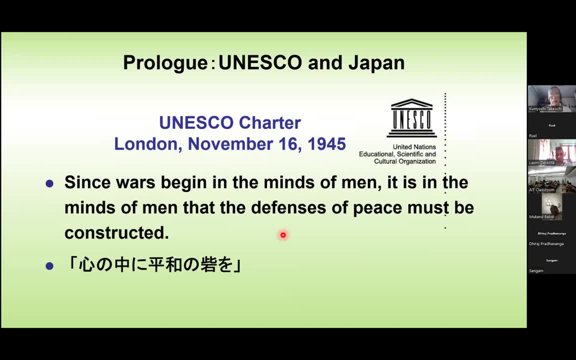 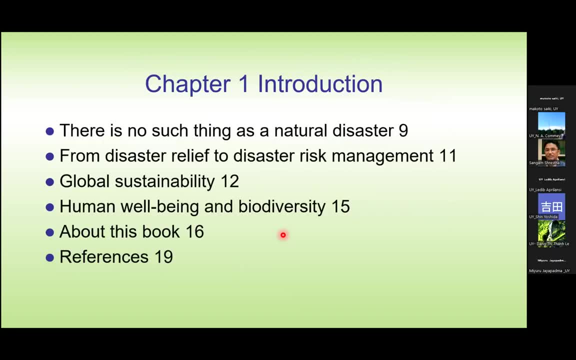 This is very important thing and this attracted me to come into UNESCO activity, The chapter one, introduction. I have not only this, no such thing as a natural disaster, but then from disaster relief to just risk management, global sustainability, human wellbeing and biodiversity. 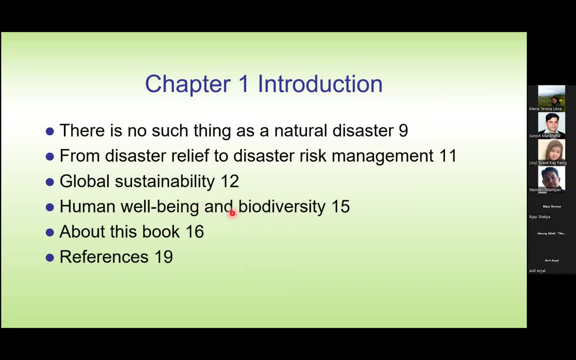 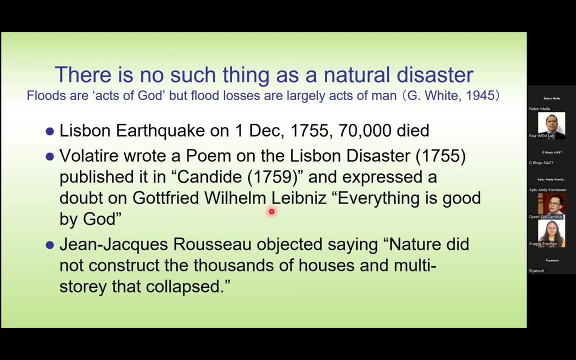 This is actually the objective of of UNESCO research, all activities, human well-being and biodiversity. well, there is no such thing as a natural disaster. you may have heard about the frauds acts of god, but the fraud losses are largely acts of men by gilbert fight. but this kind of idea started from uh lisbon earthquake? well, started in western 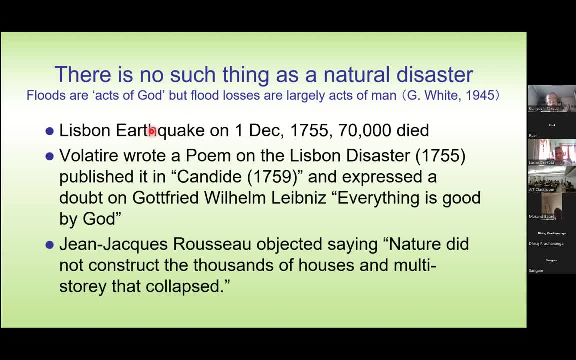 uh, you know culture uh, the lisbon earthquake uh on uh in 1755 and the? uh french uh the philosopher and the russo you know the janja crusoe, or their communication? uh made this idea first. the janja russo said: nature didn't construct the sounds of thousands of houses and the multi-story that. 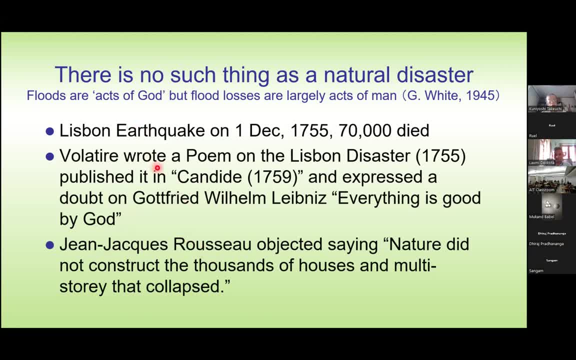 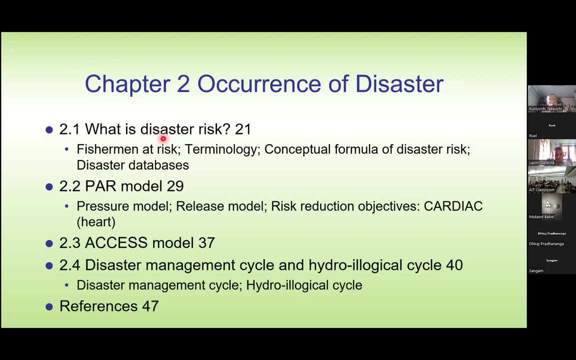 collapsed, in other words the janja crusoe, or said god did something wrong, but the janja gruesome said: it's not a matter of god, it's a human. so this story will i introduce in in my book. in chapter two i talk about what is the disaster: risk and power model i mentioned, and access model and the 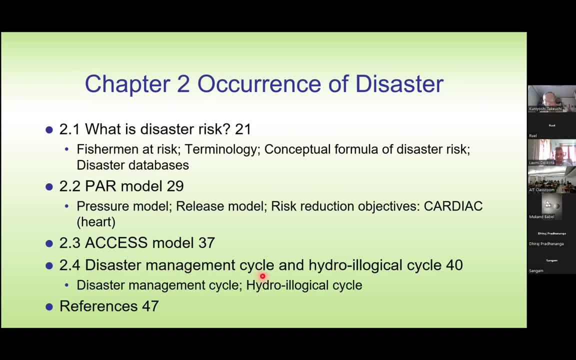 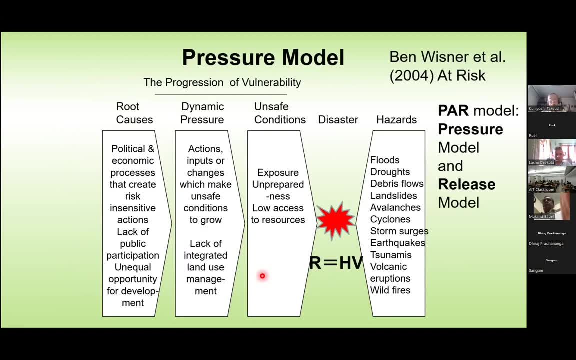 disaster management cycle and the hydro illogical cycle, hydrological. you may be interested in this. well, i have no, not much time so so i introduced just pressure pressure model. pressure and release model is about the, the, about disaster risk. it's a combination of hazard times, vulnerability, 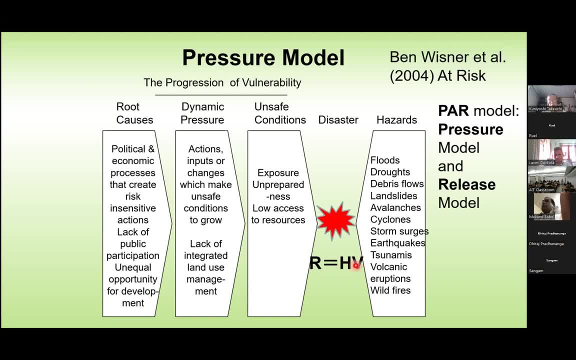 When the hazard meets with societal vulnerability, a disaster occurs. I'm sorry, In this book- it is Ben Wisner's and Pierre Braque's book At Risk. they consider vulnerability is not just unsafe conditions in front, but there is a root causes. 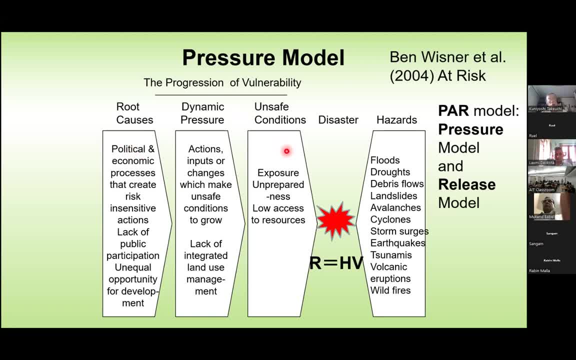 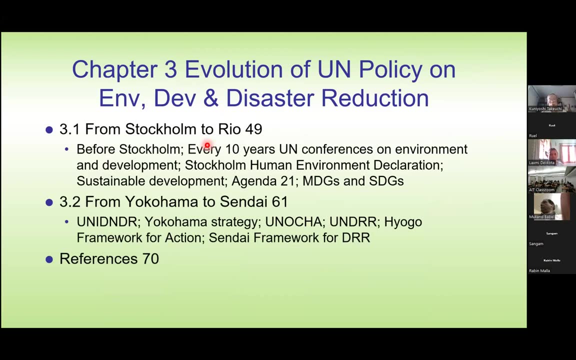 and between root causes and unsafe condition. there is dynamic pressure to translate root causes into unsafe condition. This has been discussed in the book, Chapter three, evolution of UN policy on the environmental development and disaster reduction. As I said, it is important to review the conceptual. 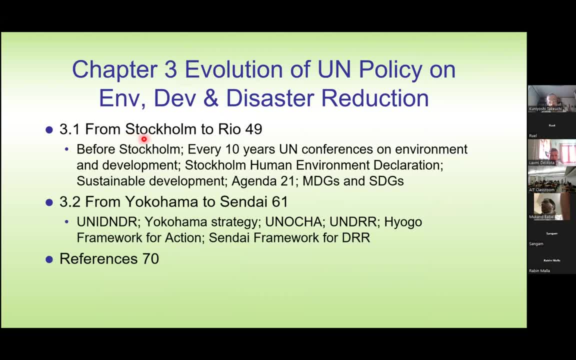 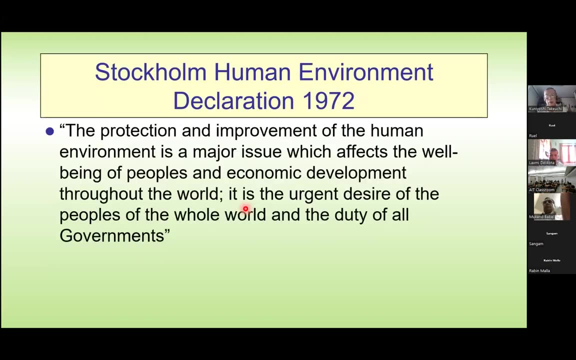 and policy evolution from Stockholm to Rio and from Yokohama to Sendai on the disaster reduction. Well, Stockholm human environment declaration was in 1972, and this, this is the declaration said: the protection and the improvement of the human environment is a major issue which affect the well-being of peoples. 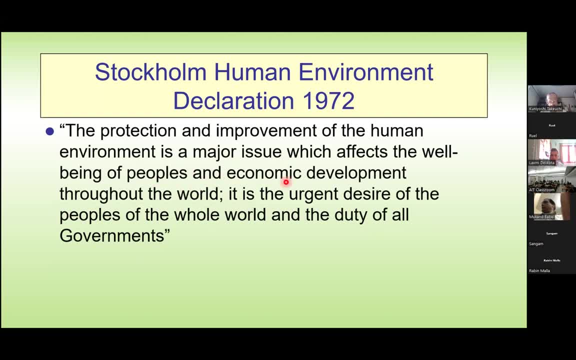 and economic development throughout the world. It is the urgent desire of the peoples of whole world and the duty of all governments. and it was very fine And it was a historical and controversial issue still today. Thank you, It was accepted by many countries in the world. 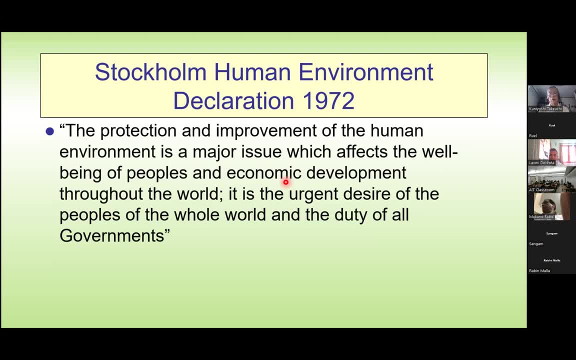 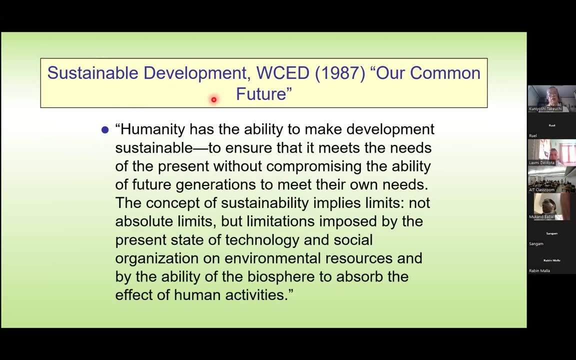 However, this statement was more like for advanced countries And the developing countries need development first rather than environment, And this conflict led to this sustainable development idea by World Commission on Education and Development 1987. And you may know it is quite important. well famous definition of sustainable development. 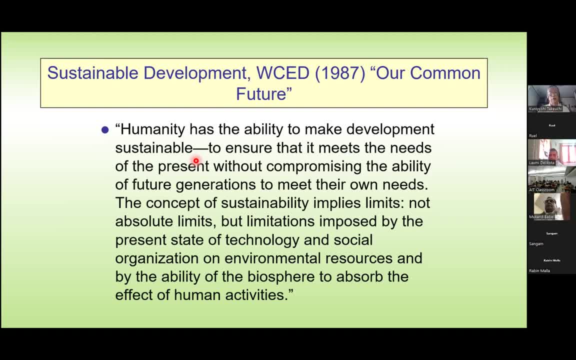 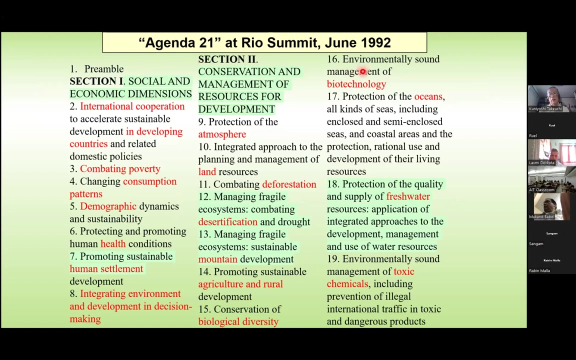 which is humanity, has the ability to make development sustainable, To ensure that it meets the needs of present without compromising the ability of future generations to meet their own needs. Well, this is quite influential, the basic policy of UN activities, And they put on this Agenda 21, 1992 at Rio. 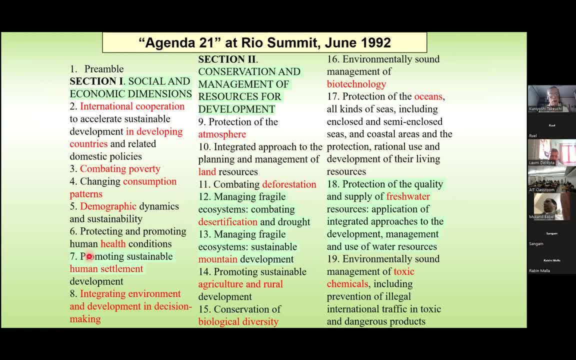 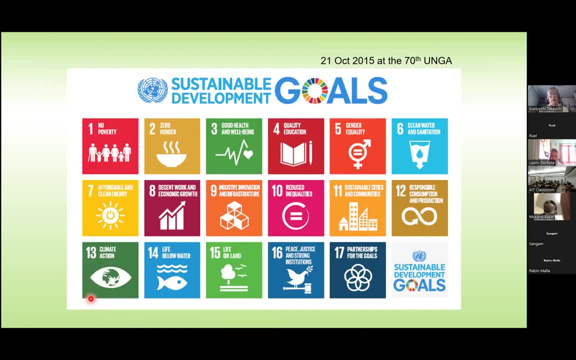 And the About the disaster. promoting sustainable human settlement was the most important one. Well, that led to our recent sustainable development goals, SDGs. Well, we had MDGs- Millennium Development Goals- first, But now this is the kind of story. 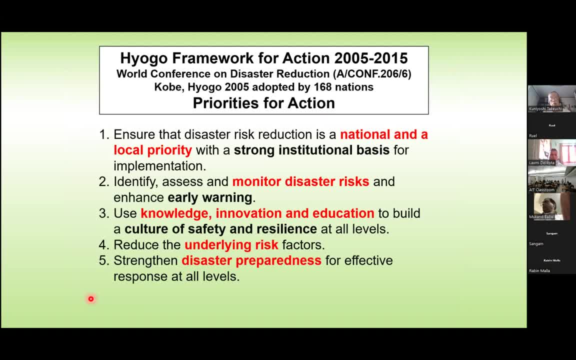 And then we have Hyogo Framework for Action And the Sendai Framework for Disaster Risk Reduction recently. And the important statement of Hyogo Framework for Action is ensure that the disaster risk reduction is national and local priority See With a strong institutional basis for implementation. 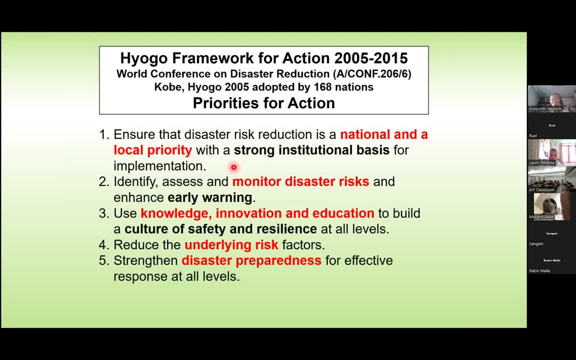 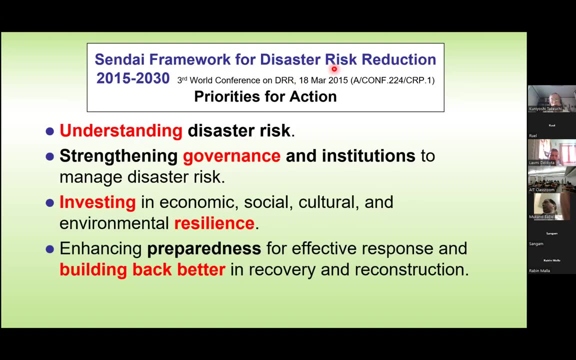 All the countries agreed on this. That's the priority, The national and local priority. We should put priority on this And we have reached in 2015,. this is a Sendai Framework And the Sendai Framework is not a kind of revision of Hyogo Framework. 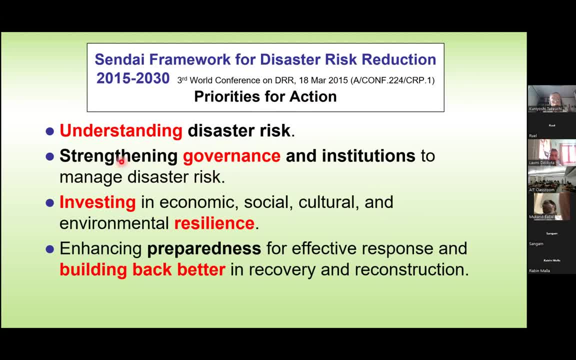 But this is a strengthening of the Hyogo Framework. The understanding is a science And the governance you know investing in the economy And the resilience came in And building back better. This is very important. Building back better was not in this Hyogo Framework. 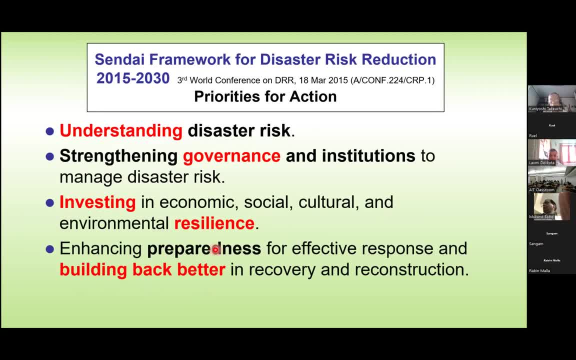 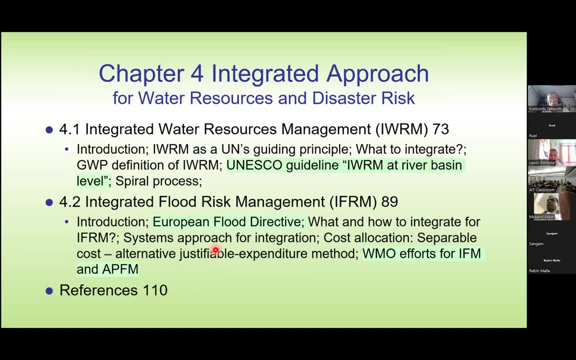 And building back better came into the Sendai Framework. Okay, Chapter 4.. Well, I'd like to have your questions. I should be very fast. The integrated approach. Well, integrated approach is for water resources and disaster risk. Well, integration nowadays is considered as a kind of the conclusive. 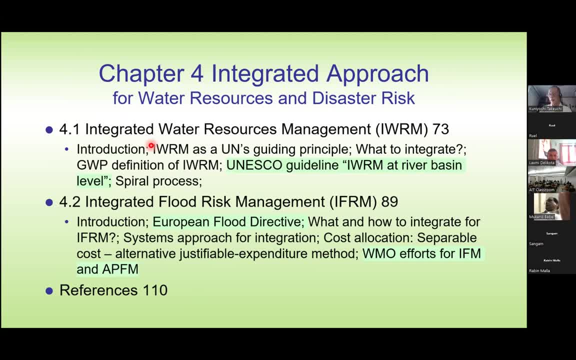 well, the most important method to proceed, the interdisciplinary problems So, and this one, integrated water resources management and integrated flood risk management. And we have UNESCO guidelines And the UNESCO European Flood Directive And WMO efforts of integrated flood management. They are kind of examples. 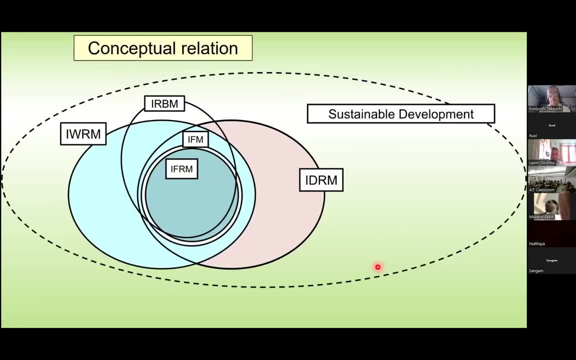 First, I consider integrated flood risk management is in the center of the. it's a part of integrated water resources management and integrated disaster risk management, And they all contribute to sustainable development, See, And this relation is quite important. So, in other words, 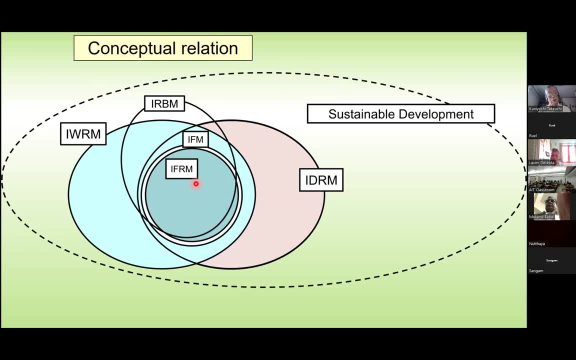 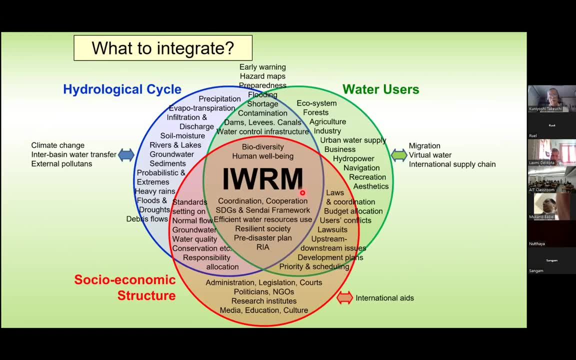 integrated flood risk management is part of integrated water resources management and integrated disaster risk management. We shouldn't make this. this is separate. Well, what to integrate? Of course, integrated water resources management, hydrological cycle, water users and the socioeconomic structures. 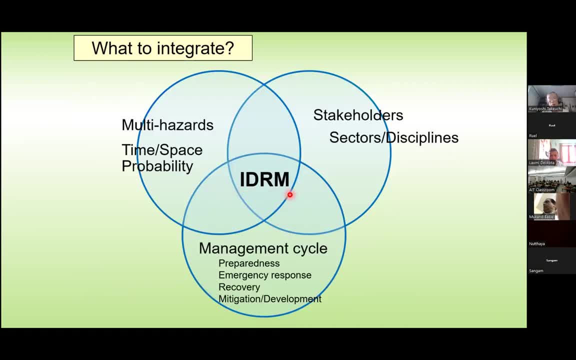 Then what is integrated disaster risk management? We should integrate multi-hazard and all the natural characteristics- time, space, probability- And also we have users, stakeholders And the management cycle. They are more like processes of disaster risk management. 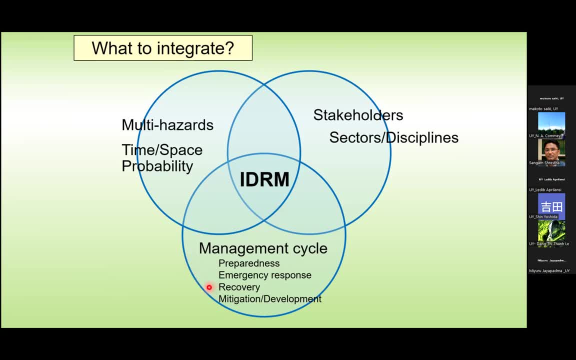 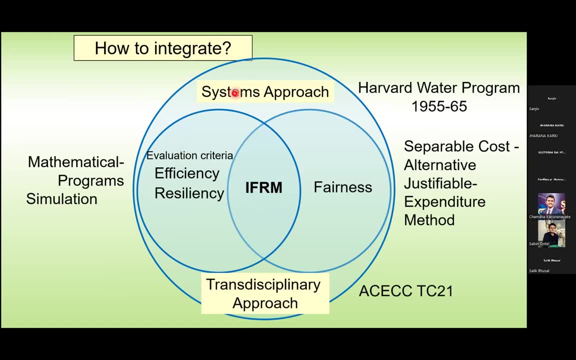 Preparedness, emergency response, recovery and mitigation. Well, how to integrate? You may know systems analysis approach and the trans-disciplinary approach. Now, as an example, there is all the but the very important: the initiation made by Harvard Water Program. 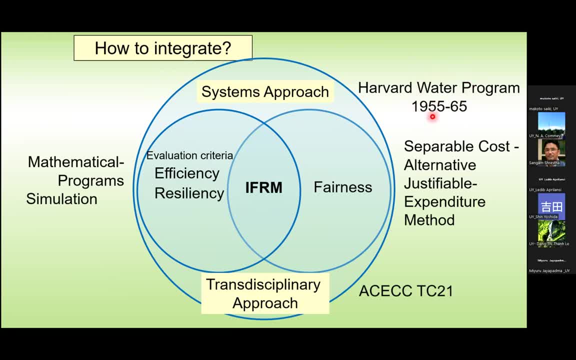 more than half century ago, But they produced a book: Design of Water Resource Systems. It is considered as a bible of water resources. So this is briefly, very briefly introduced And integrated risk management. it is necessary to have efficiency and fairness. 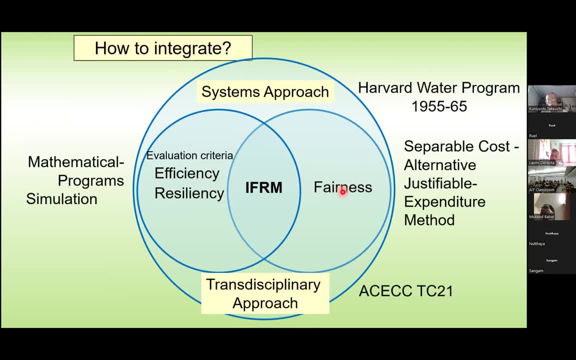 Efficiency or resiliency and fairness And as an example, separable cost alternative, justifiable expenditure method is explained And mathematical programs and simulation. this is not touched upon This, just a few lines. And about trans-disciplinary approach, I introduced ASEC TC21 activity. 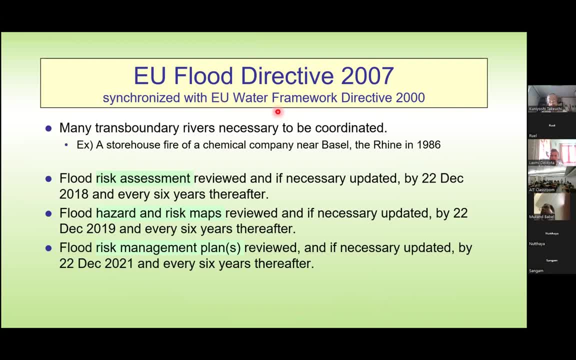 Well, EU flood directive. This is very interesting and important exercise which is part of EU water framework directive, Started 2000.. And the most important mechanism of integration of this initiative is six years. you know, every six years it should be repeated. 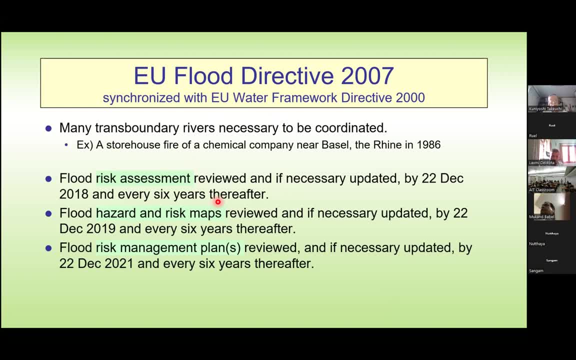 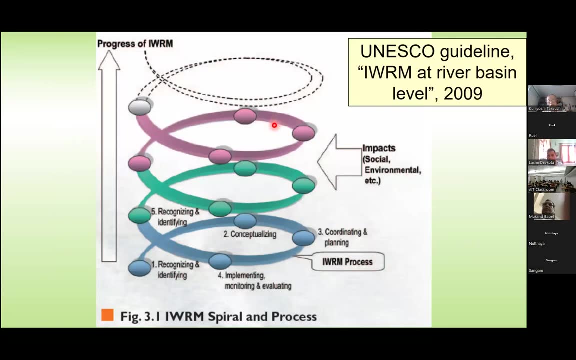 Repetition, periodical repetition of assessment, risk maps and management plan. This is quite interesting approach And this has been explained in the book And the UNESCO guideline IWRM. it's about this spiral, spiral process, Because each society has different development levels. 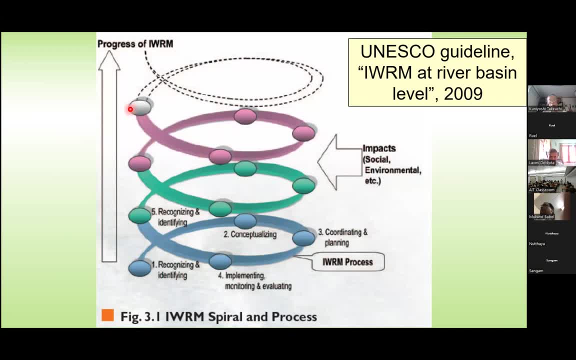 Therefore, IWRM faced many challenges And I think that IWRM should also be upgraded step by step And in those the stepping up, there should be some occasions, And those occasions step up occasions are most often it is a disaster. 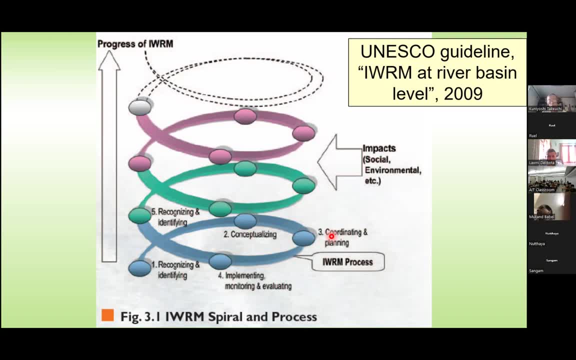 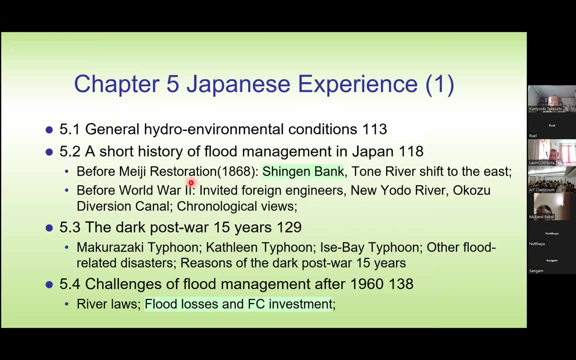 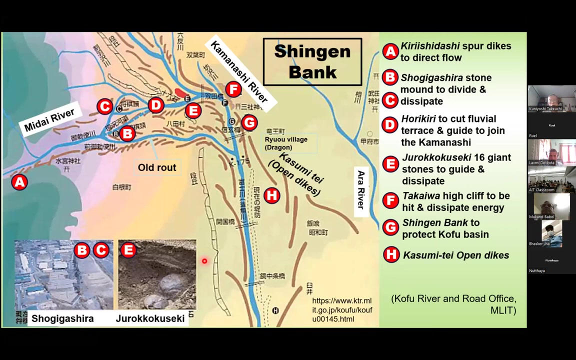 So disaster is opportunity window To say see the, this opportunity window to use opportunity window. Well, chapter five, Japanese experience. I have start from the general hydro environmental conditions. This is not nature. And then the history. Then the history includes: 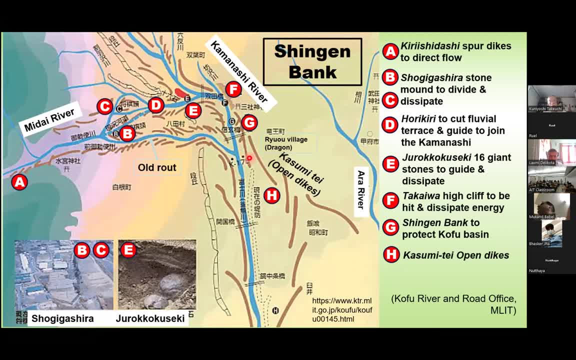 this Shingen Bank which is in Kamanashi River, of Fuji River, in my place, And I like to say all of my students at ICHAM or the, the Malaysian, the University of Technology, Malaysian student, come to. 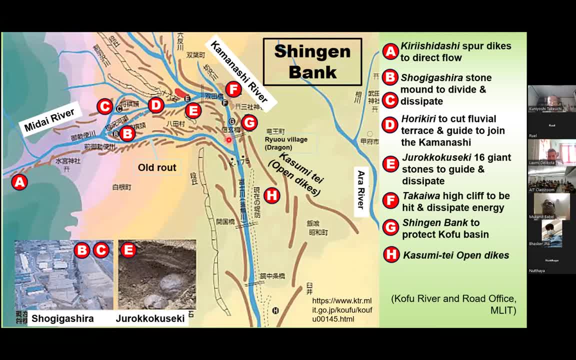 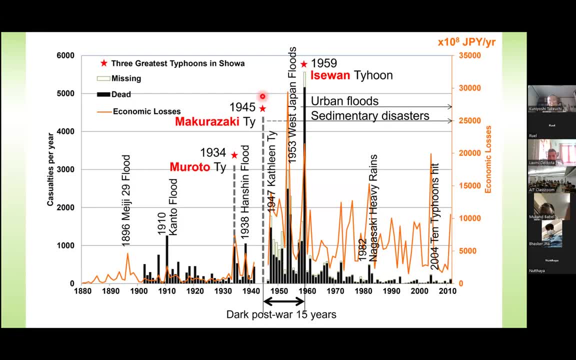 my place and see the historical Shingen Bank And I like to. this has been also quite explained. And then the history- it says Japanese- the flood losses And in 1959, more than 5,000 people died in. 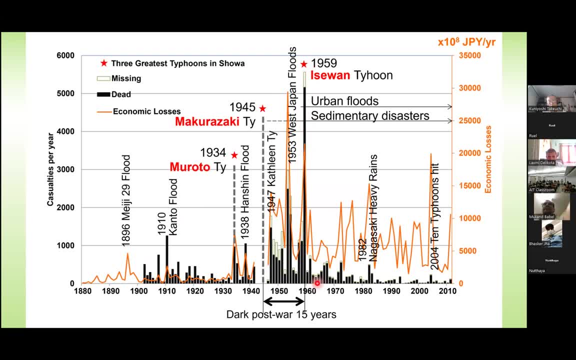 Nagoya area by storm surge And this is considered this- 1945 to 1959, is considered dark post-war 15 years And this is influenced by the defeat in the war. In other words, war made this the dark post-war. 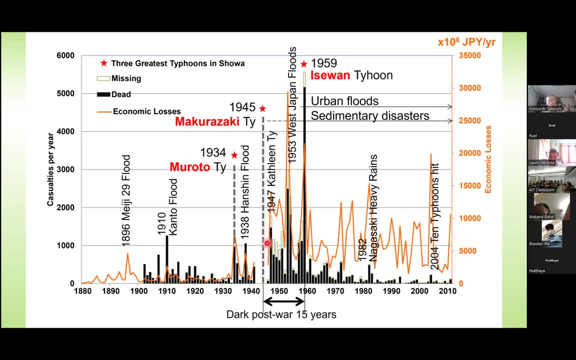 of 15 years. But it is important to say, after that the Japanese, the death tolls declined and declined, But the red one means the economic losses. And the human losses may decline, but not economic losses. This has been also explained. 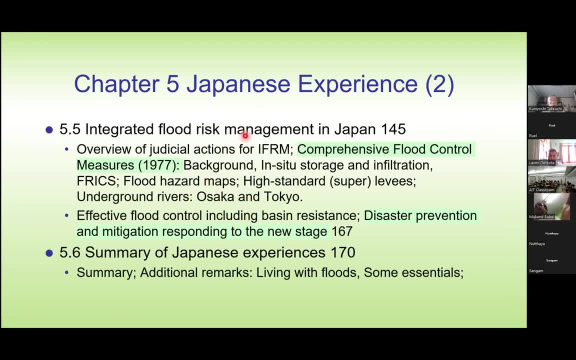 And second part of Japanese experience is about the, about the current, current flood risk management, And the current flood risk management is comprehensive flood control measures and disaster protection and mitigation. responding to the new state- And I'd like you to know, the 1977,. 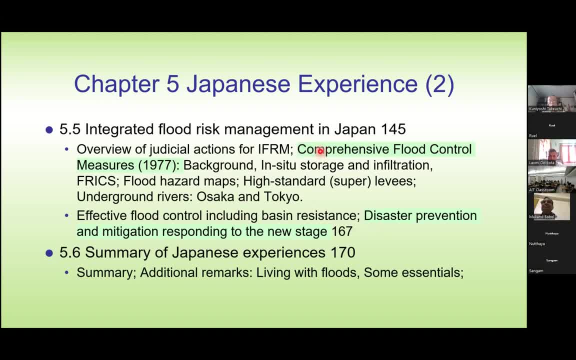 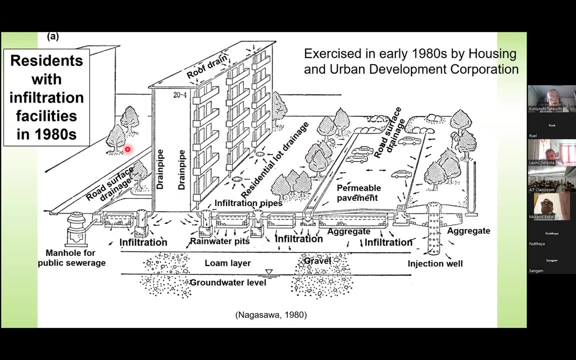 this is actually the sponge city idea. Sponge city idea is a new one, but it is much before Japan started And this is one of the sponge city idea for residents with infiltration facilities. It is already known. It is already 1980s. 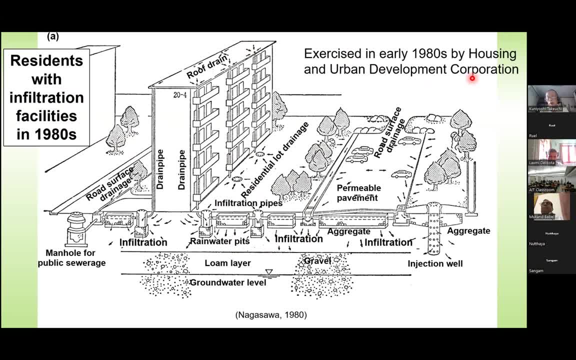 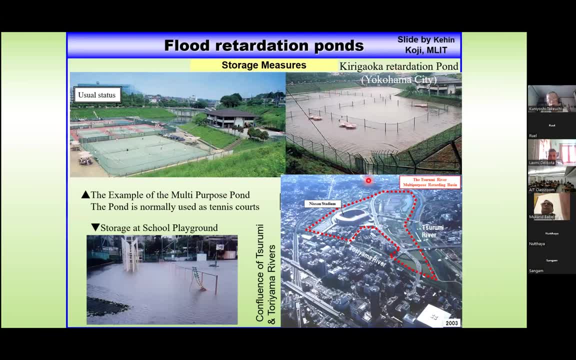 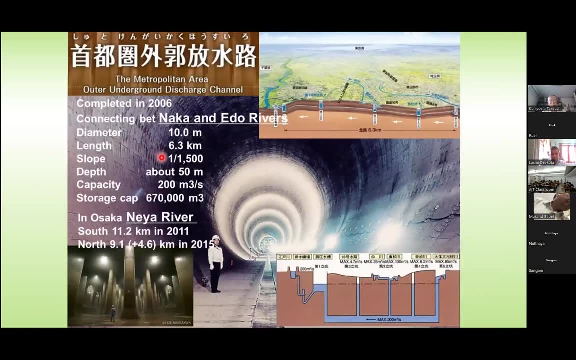 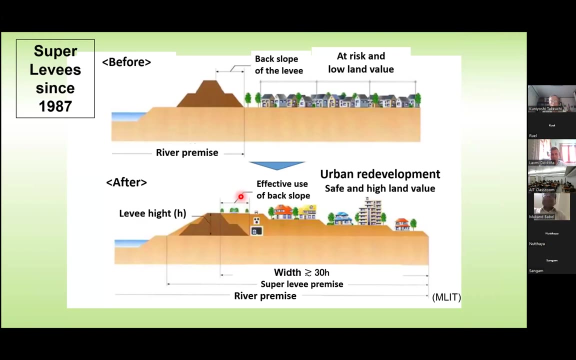 in the, in the urban development corporation- you know public corporation- And the. we have the storage, even the, the playground is used for storage And of course we have such as the underground rivers and super levees, And they all are. 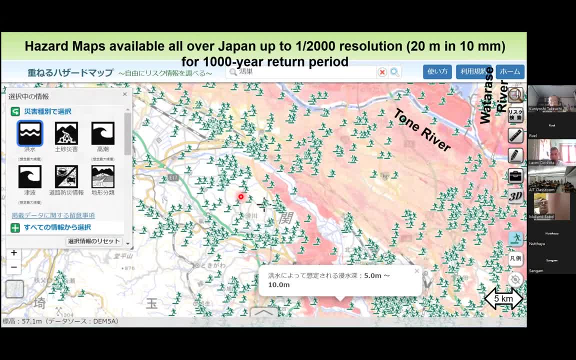 quite much explained And now we have hazard maps, And I like to say this hazard map is available all over Japan in 2000,, one over 2000, which is 20 meter in, in 10 millimeter. So that is why. 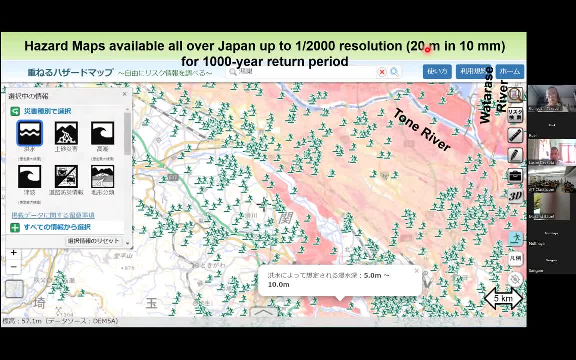 we can see even my house in this map And this is for 1,000 year return period, And that's this is for flood or landslide or storm surges, tsunamis and such, And this is warning for evacuation. 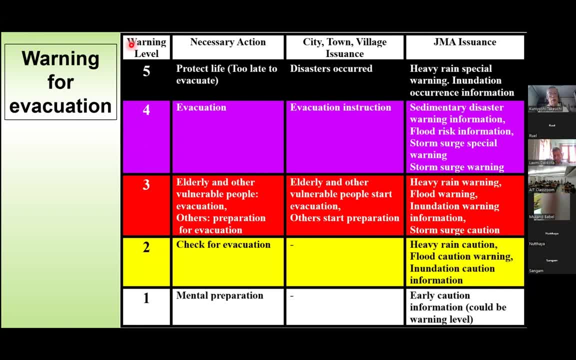 Now exercise. We have warning level five And warning level one, mental preparation, And the, the physical check for evacuation. Number three: elderly starts and other vulnerable people starts evacuation and other prepare evacuation. And the number stage four: it is evacuation. 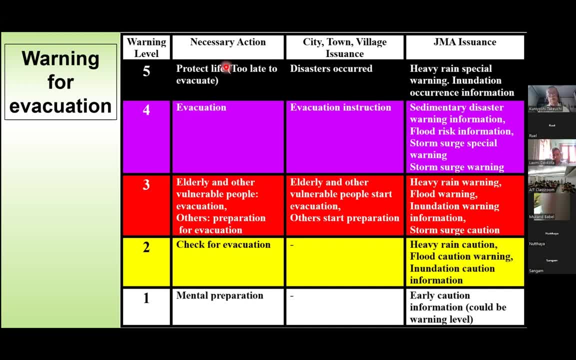 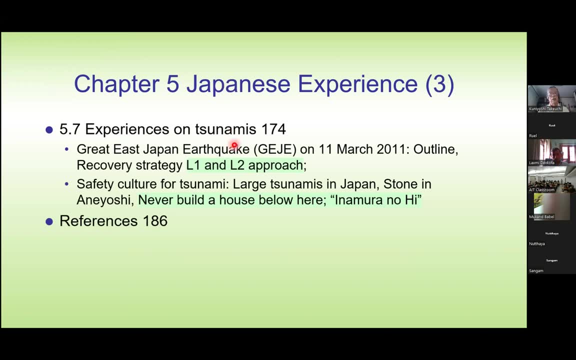 all people And the number five it is disaster has already occurred and people shouldn't move now It's too late to evacuate. This is the what now exercise in Japan, And the final part of Japanese experience was experiences on tsunami, And we have. 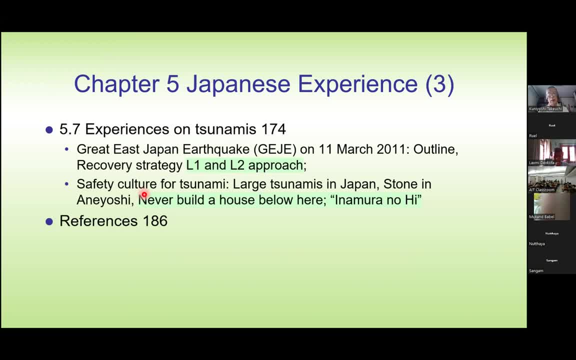 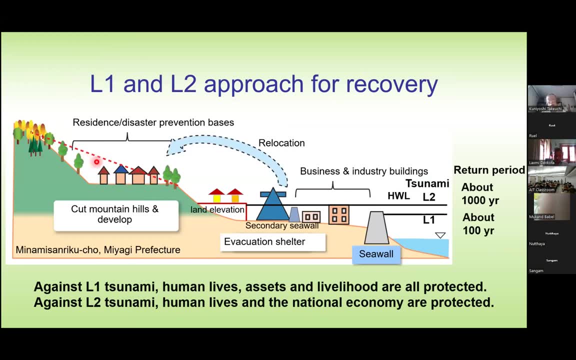 L1 and L2 approach and some culture for tsunami. And L1 and L2 approach is: L1 tsunami is considered about 100 year return period, For for that every tsunami should be protected by physical facilities, And about 1,000. 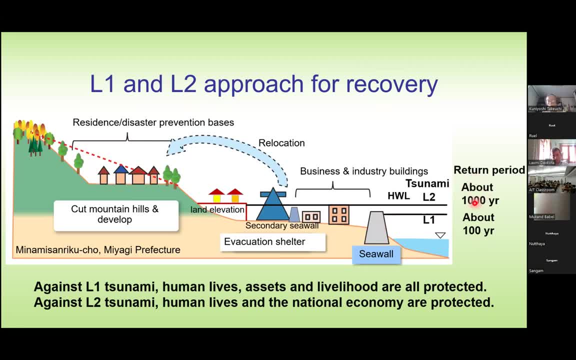 year, that is, L2 tsunami. This should be protected only only human lives and national economy. So people has to move from here to somewhere up up. That is why the Japanese, the Japanese. the recovery of the Tohoku tsunami was quite late. 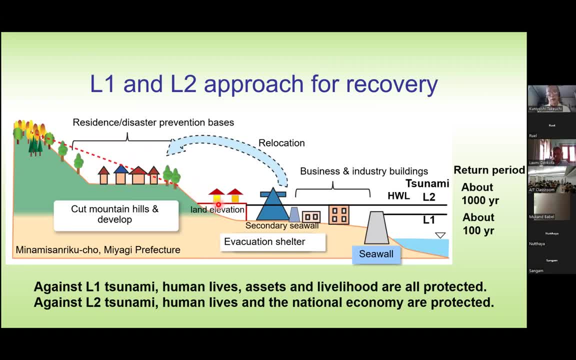 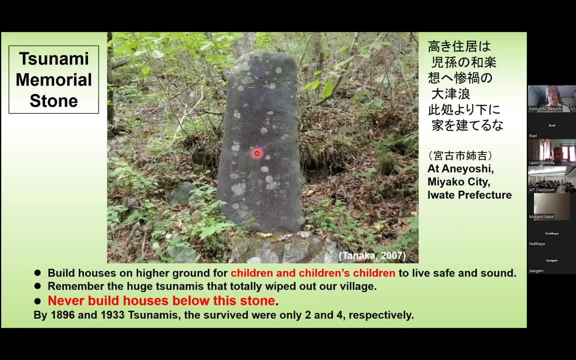 And even now it is the people are working on And this is tsunami memorial stone in Miyako, And this says: never build houses below this stone. And this is the story of the tsunami that was struck by tsunami 1896 and 1933. 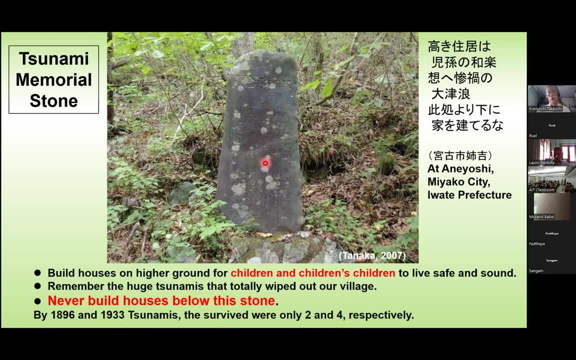 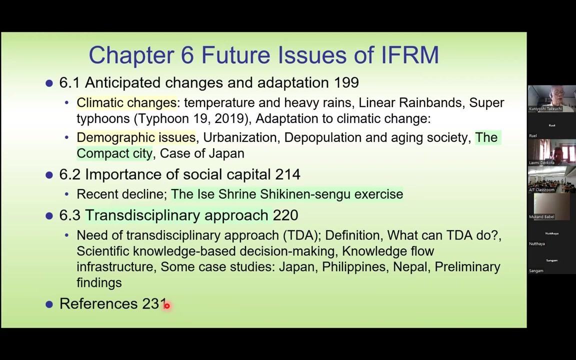 twice, And only the survived were two and four people. That is why this stone was put on the US border as a representative of the tsunami that was struck in Miyako, And this is the story of the tsunami and the impact that this 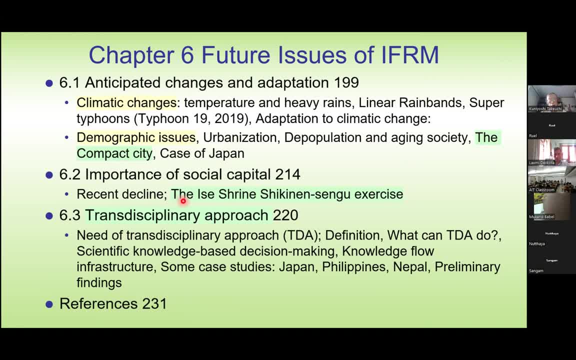 tsunami has had on need social capital and social capital for Ise Shrine, the Shikinen Sengu: 20 years rebuilding for 800 years, 20 years rebuilding has been continuing. So this was introduced and transdisciplinary approach by, I said, ASEC, TC21. 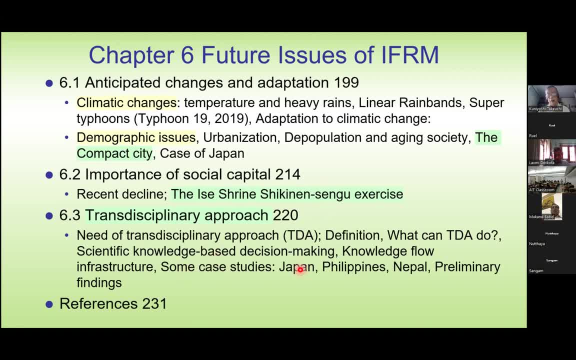 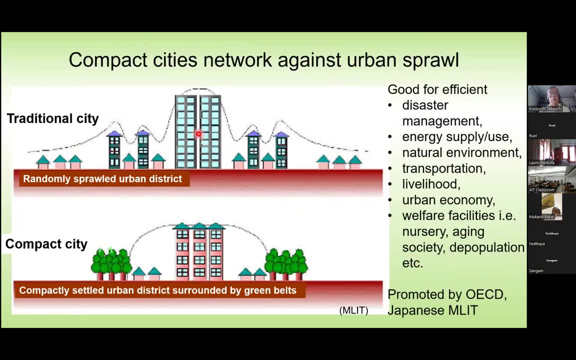 And some case studies- Japan, Philippines, Nepal- and the preliminary findings mentioned. Well, compact city, the city with sprawled urban district- is very inefficient and very bad for disaster management and the environmental condition and the economy too. So put it into compact city. 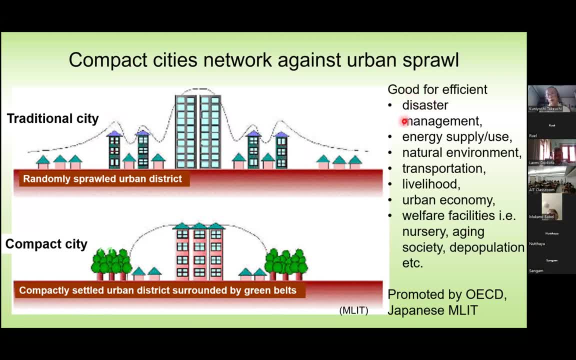 Then this is good, very efficient for disaster management, energy supply, natural environment protection and transportation, livelihood, urban economy and also welfare In the aging society. we do need the hospital, the aging society and the district. The population needs those places. 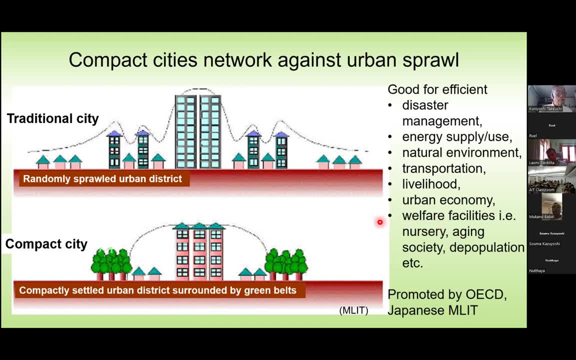 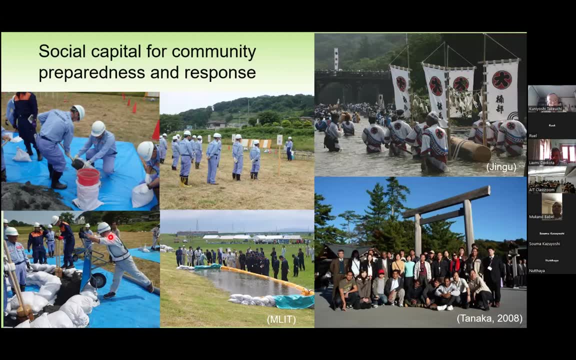 And the compact city is very good. Well, the other thing is, in order for the preparedness and response, we do need community activity, And this kind of thing shouldn't be only by disaster training, But it should be by- And this is the Jingu Shrine- 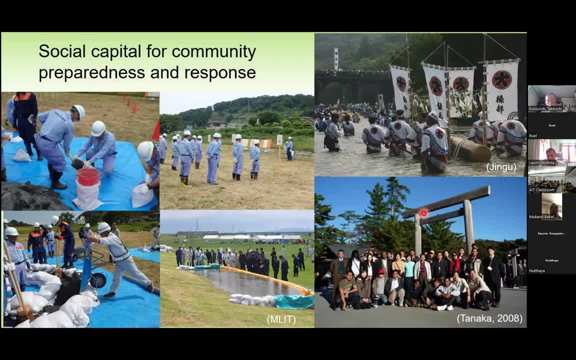 I said I'm sorry I cannot explain, but 20 years, Every 20 years, rebuilding of the shrine, And then the people has to work together like this, See, Like this. And 20 years, 800 years, it is continuing. 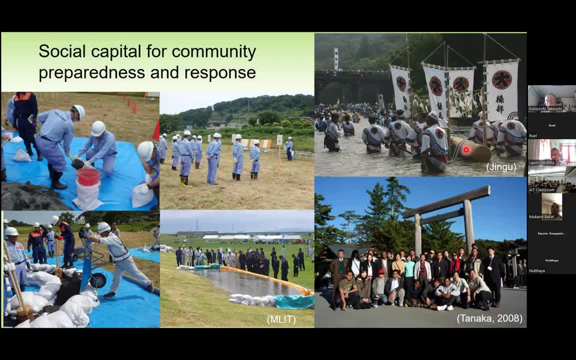 That is why, for instance, this: Yeah, Yeah, Yeah, This wood should be kept in the forest. If there is no forest, then they cannot be built, And not only just a building, but also some decoration too, using the feather of a bird. 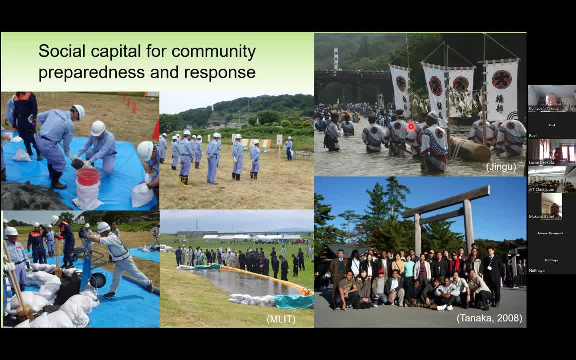 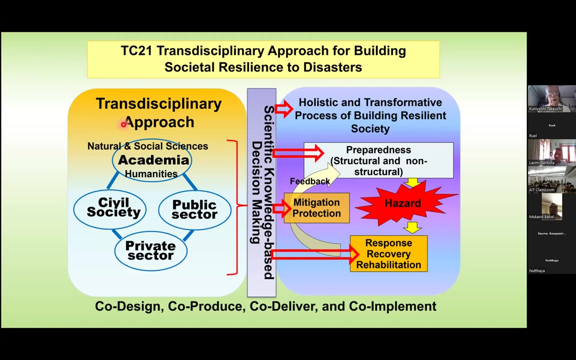 And if that bird, that is a special bird called a toki, we can rebuild it that way by building it. So, for example, if Toki disappears, then we cannot remake it. So this kind of rebuilding every 20 years continuously is a very, very important sustainability exercise. 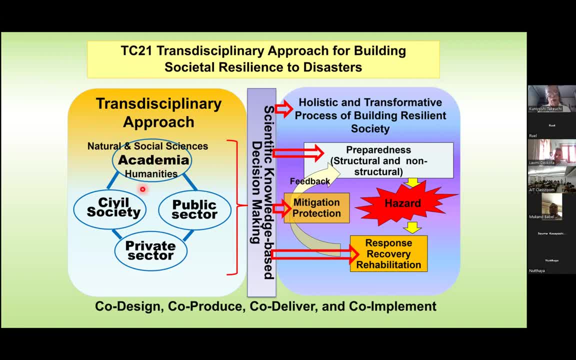 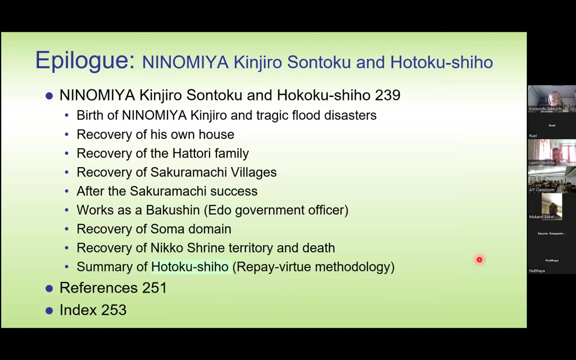 society, public sector and private sector all together. we work through scientific knowledge based decision making to disaster management, and not only did co-design and co-produce, but also could deliver and co-implement. so even students uh, nowadays, are requested to come into the implementation. uh the the interest, okay, uh epilogue is: uh ninomiya uh kinjiro stontok. well, 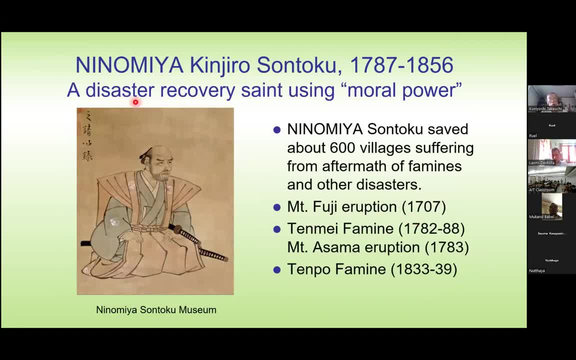 uh, he is, as i said, a disaster recovery saint using moral power. moral power, see, he. he lived the 1787 to 1856. we had quite much of the famines and the great eruption, of the volcanic eruption, and that he showed. he made 600 villages suffering from aftermaths of famines and other disasters. 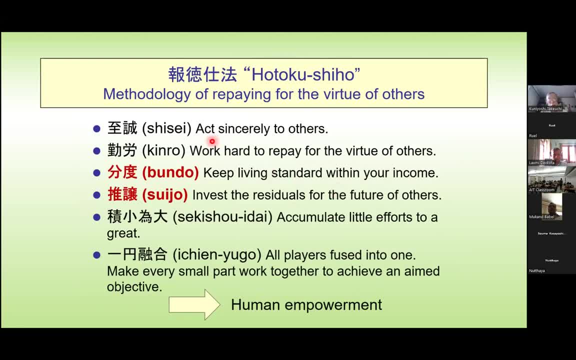 well and his method is: uh actors since the six uh the act sincerely to others, work hard to help theme within the world. uh uh. third, uh uh to residuals for the future of others. Invest residuals for the future of others And accumulate little efforts to a great. 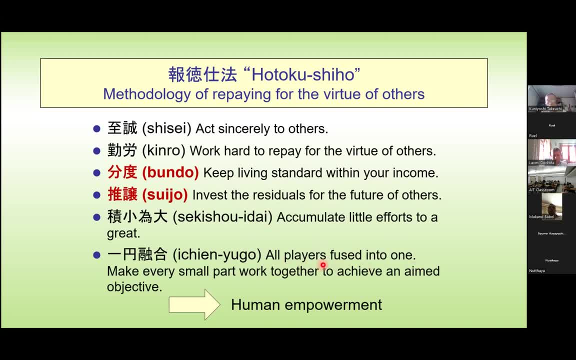 and all players fused into one. See, all players fused into one. This is transdisciplinary approach, Okay, And all of this is a moral, is not only just a discipline, but moral is real power. It is an economic power and also any kind of basis of the development. 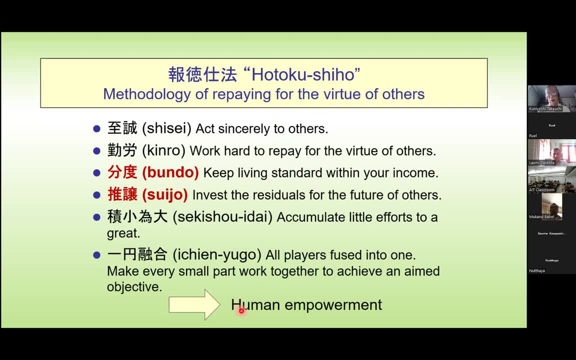 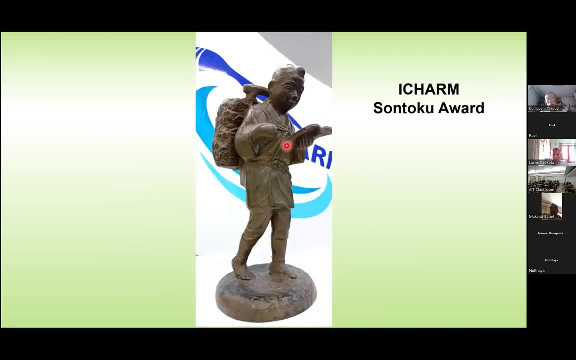 And this is as a whole, is considered as a human environment empowerment. Well, at IHM we have so-called Sontoku Award, which gives the certificate and also the statute- miniature statute- of moral and economic power of moral and economic power. 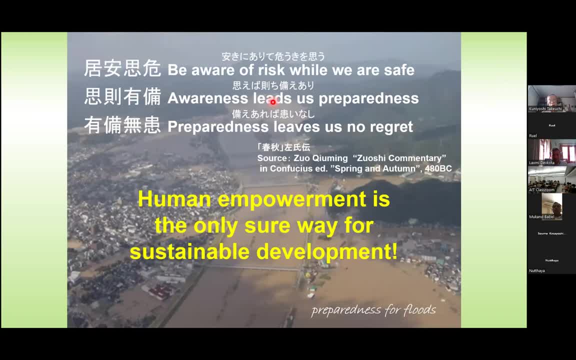 Well, this is the last slide I always give you at the end of my lecture. I always give you at the end of my lecture, which is the 2,500 years old Confucius saying. which is the 2,500 years old Confucius saying: 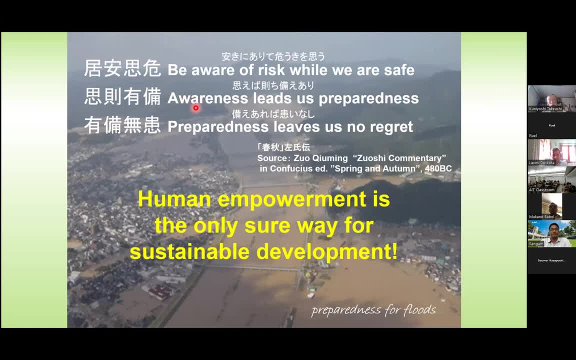 be aware of risk while we are safe. Awareness leads us preparedness, and preparedness gives us no regret. And the most important statement I like to leave you is: human empowerment is the only sure way for sustainable development. This is repeatedly mentioned in my book. 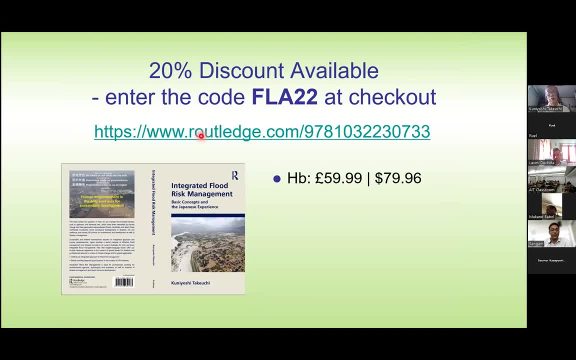 Okay, The final one is this: 20% discount available on this book. It is too expensive, actually really expensive, But unfortunately there are no paperbacks. but unfortunately there are no paperbacks now. So I really appreciate if professors have a fund. 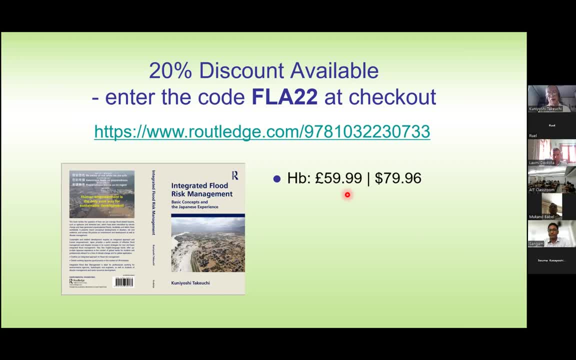 So I really appreciate, if professors have a fund, then you prepare some of those books in the shelf. then you prepare some of those books in the shelf. Okay, Thank you very much. That is my lecture. That is my lecture And I hope you have some questions. 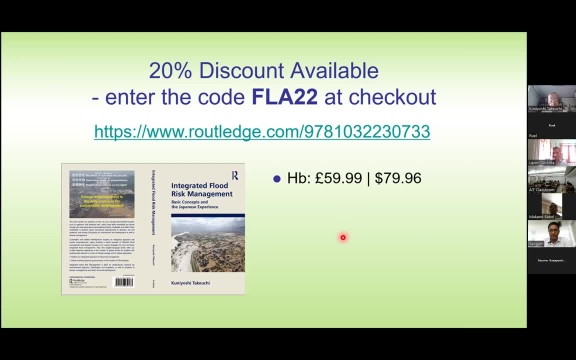 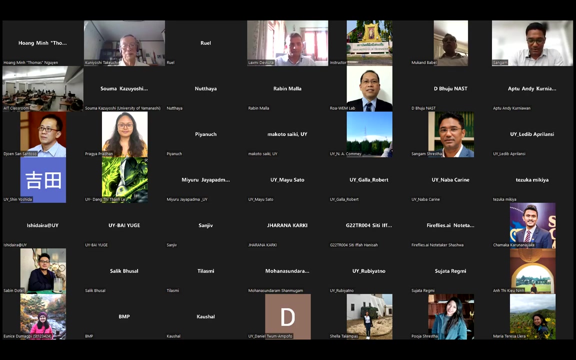 And I hope you have some questions. Yeah, Thank you, Professor Takeuchi. Thank you very much And you know that you have brought you know lifelong experience of this flood risk management in the book. And, once again, congratulations. I have already, you know, placed order one week ago. 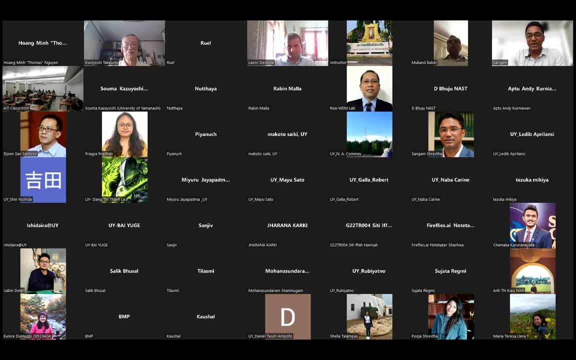 Once you had sent me email. I hope I will be getting that book next week. I hope I will be getting that book next week And I will try to keep one book in the library and also, you know, provide to my students here. 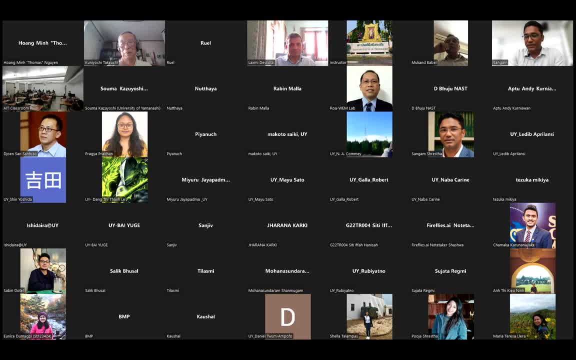 Thank you very much. Yeah, we have about 10 minutes for Q&A session And I'm sure there are a lot of questions to Professor Takeuchi, So I would like to request to raise your hands and unmute your microphone, if possible. 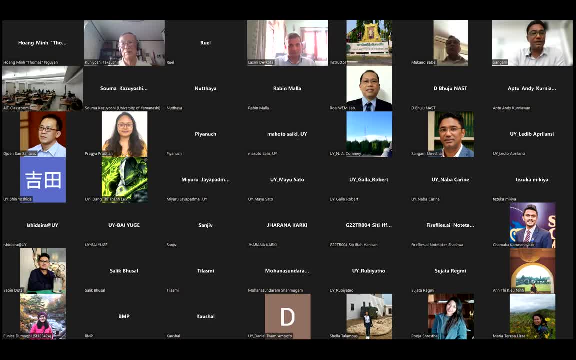 please switch on your video. switch on your video camera and you can direct your questions to Professor Takayuchi. I see one hand, I think, from our student in our classroom. Okay, Thomas, You can briefly introduce yourself right and ask questions. 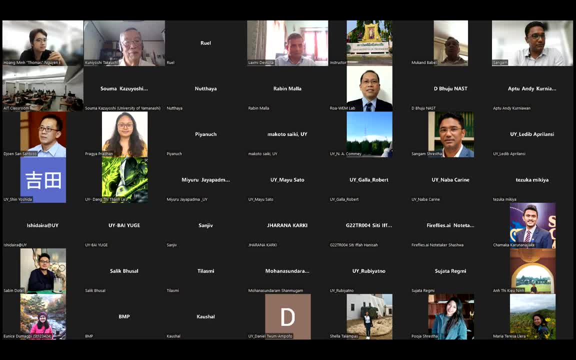 My name is Thomas and I'm a PhD student here at AIT. I have a couple of questions, but before I ask you my questions, I would like to say thank you for your very interesting introduction. I spent a couple of years in the US and I was actually 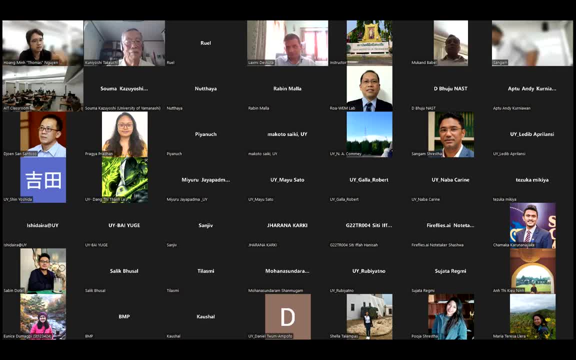 a Hurricane Harvey survivor. It hit directly my city in the US. Oh really, Yes. So my question to you is: the experience you share and the projects that you introduced were mostly related to the Grad-related disasters, Correct, Including- Yeah, mostly related to the developing countries. 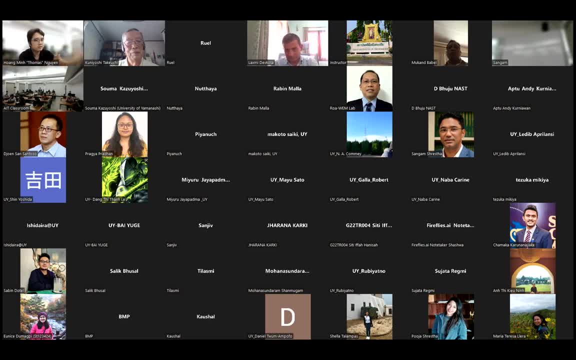 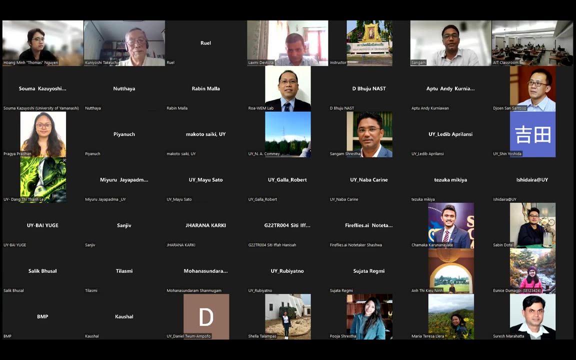 However, for a country like the US, they have a lot of money. However, every single time there was a hurricane hit directly to the mainland of the US, the economic loss and the human life loss are still significantly high every single time. So what kind of lessons should they learn from the Japanese experience in order to 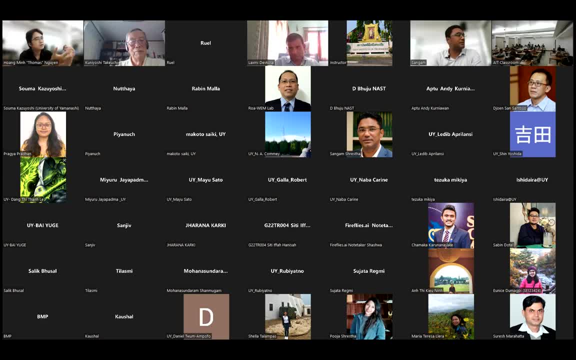 minimize their losses and improve their um hazards, protections and integrations, risk management. Well, I think my book won't be only to the European countries, but includes advanced countries, The hazard maps- I think this is really advanced in Japan- and also forecasting. 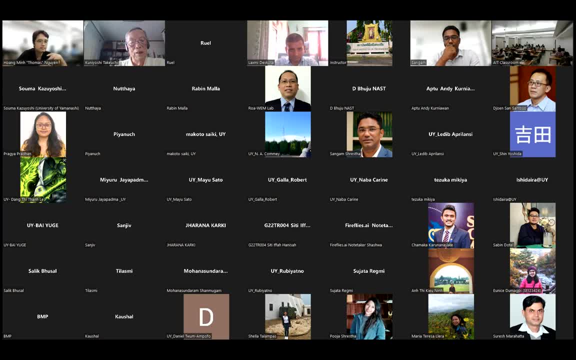 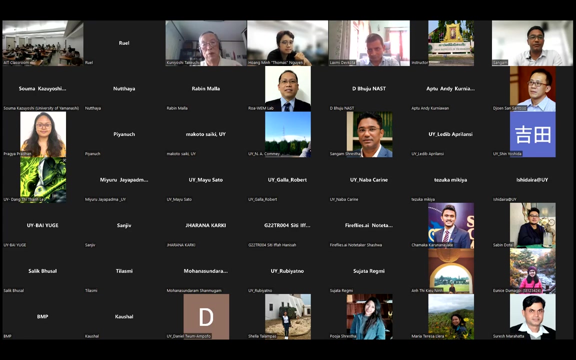 and also you know the well compact city idea. You know the in the United States it is老ad. The people are living very spread Well, but not so. so it makes very, very expensive to make some area safe. 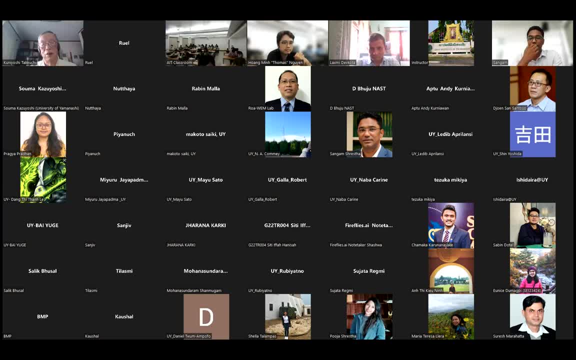 But now, for instance, in that that I said, L1 and L2 approach and Japan is now coming into L2 approach, one thousand, the return period, space, And well, people are moving into the higher place and the lower place for different purposes. 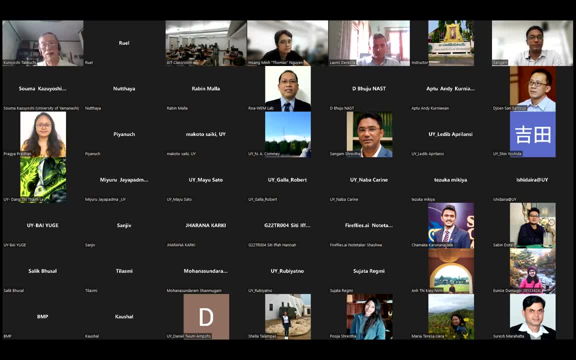 Well, I think the deep population or the increasing population, the same. the compact city is supported by OECD. They suggest the all countries to do this. Well, anything else, Yeah, yeah, yeah, good, good, Oh Well, Sangam, I don't hear. 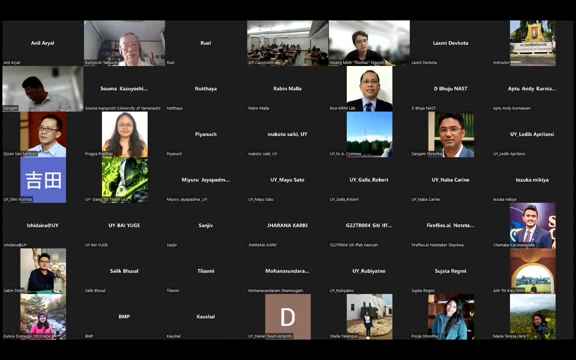 Yeah, I don't hear your. Can you hear me? Yeah, Yeah, Okay, I see one hand: Anil, Dr Anil, yeah, please, Hello Doctor, we can hear you. Yes, yes, please. 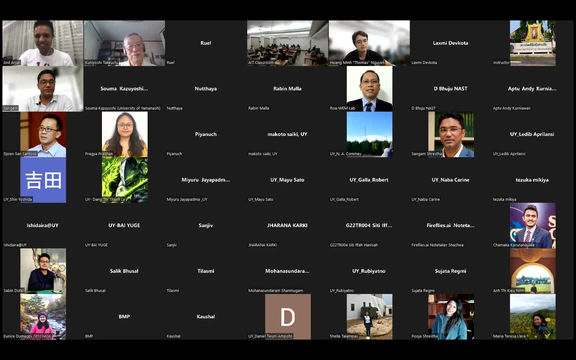 Yeah, nice to meet you, Doctor, and thank you for writing books for us. excellent was really impressive. my question is: you talked about how to integrate iwrm, ifrm and ifm. do you have an idea when to integrate and explain when can? like before 2000, we didn't talk about iwrm. 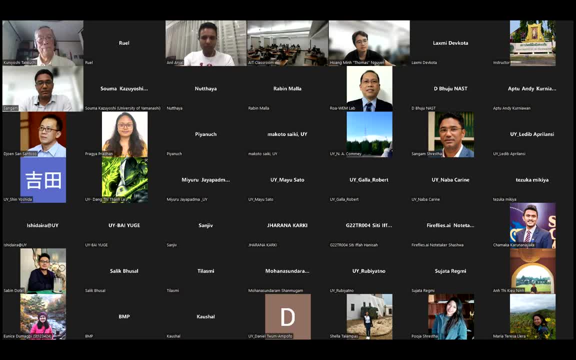 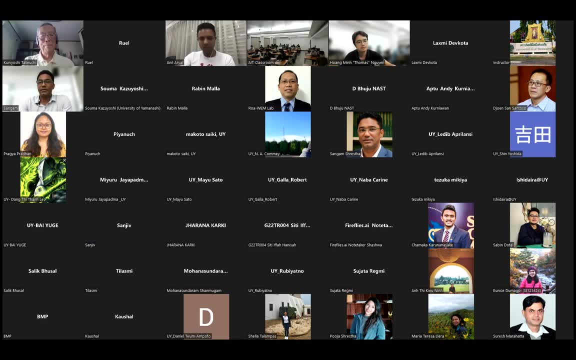 after 2000. we talked about iwrm and ifm and i and irbm. do you have a standard experience? can you explain when to integrate these terms? well, the integration is very, very impor, uh difficult, and there is no or kind of standard yet. well, of course, a mathematical approach there are. there are quite 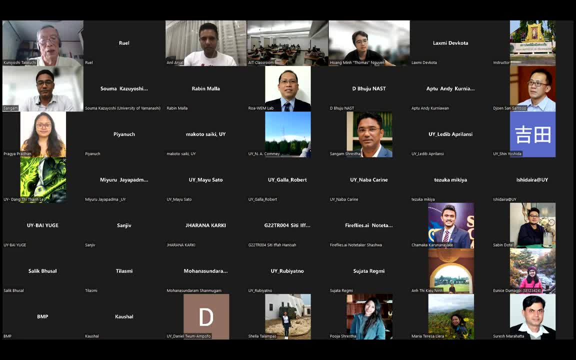 a few, the, the integration efforts. however, mathematical approach is only in a kind of focused area, where the selected components, but the, in reality, integration should take care everything you know, as i said, the nature, users and social system and the, they all. that is why transdisciplinary approach is so important. 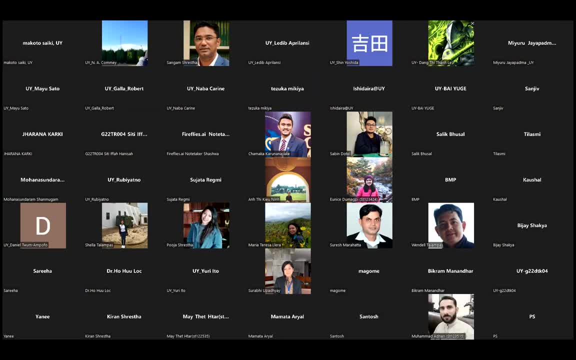 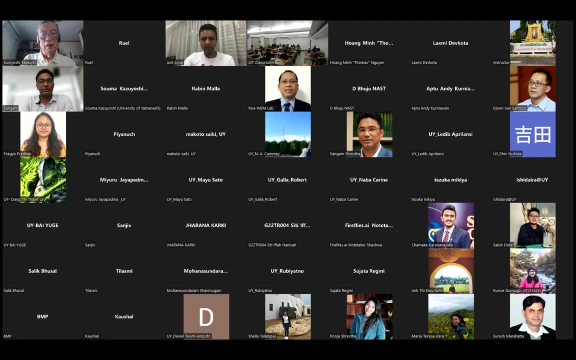 and transdisciplinary approach. uh, we, we are uh, the the promoting is, uh, the sectors, you know, sector has, academic sector, uh, public sector, uh, the private sector and social, uh. so well, civic society or community, they all should work together and then, then the it is a chaos if everybody speak. so there should be some rules, and what is their rule? that is? 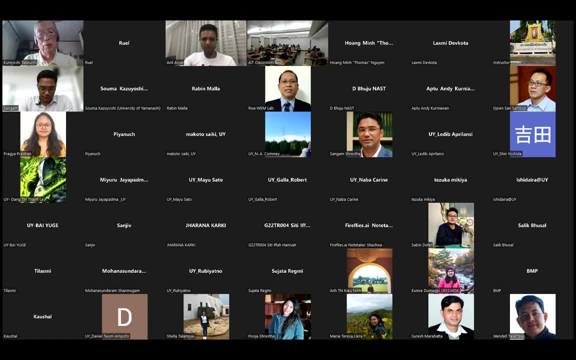 responsibility and kind of mandate they committed or they accepted. see that if we just take the responsibility on people, well, um, everybody is different right now in terms of policy direction. there is a不同 part of economy right now, and again i told you about media policy, but we need to 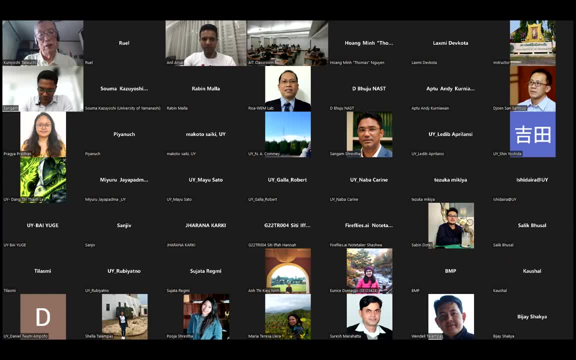 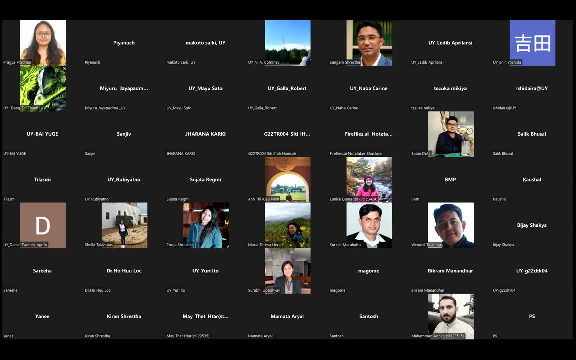 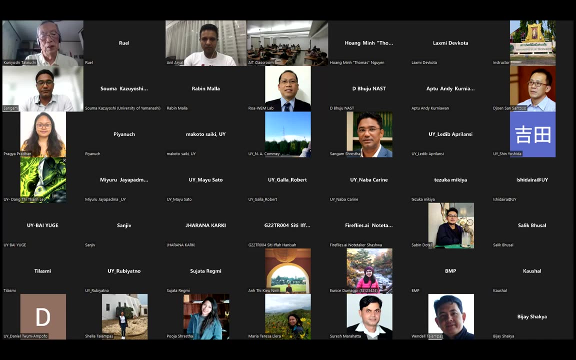 we need to a greatρίgo burden. That sort of thing has been discussed and where we are still looking into various case study area, Some Japanese case study. that is the kind of committee Whenever government faces some difficult problem which needs societal transformation and such. 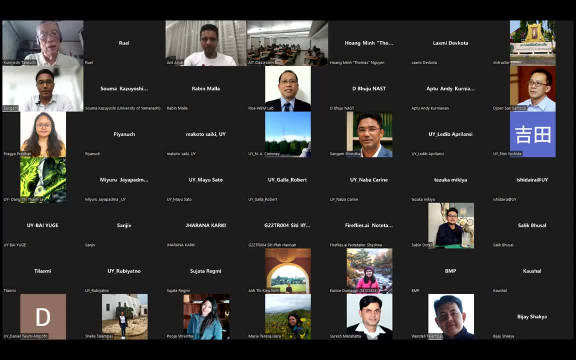 then we organize a transdisciplinary committee where the scientists and the public sector or private sectors, the civic society get together and work together. And of course this should be the multiple disciplines. The well When natural science and social science and art should work together. 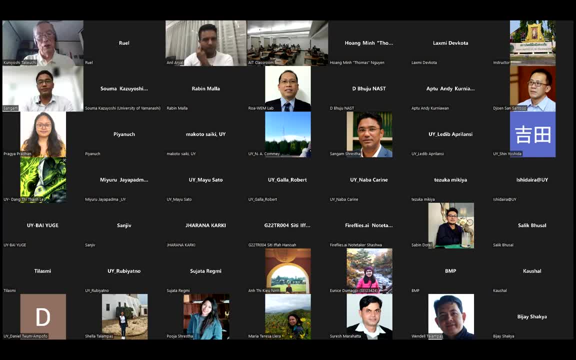 Well, this is a new area to explore. So I cannot say there is a fixed integration approach now. And governance is very important. You know, the governance in many countries, especially developing countries, are suffering from governance issue. Well, that is everybody's note. 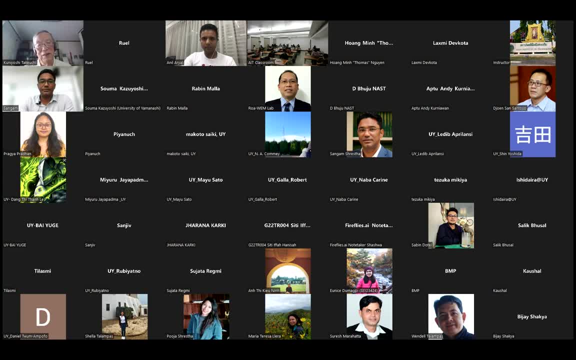 Well, thank you for your question. You may like to ask something else. Yeah, thank you, Professor Pakiewicz. I think there is one question from chat box. This is from Dr Denise Wuzhu from NASS. So the question is: 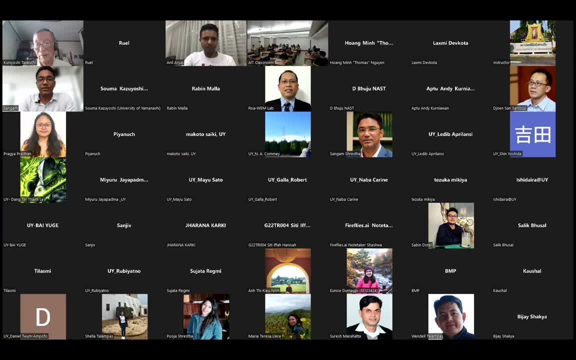 is disaster preparedness a human awareness or technological approach? I'm reading question from Dr Wuzhu: Yeah, yeah, Well, thank you very much. The disaster preparedness is very important. I don't say this is just human awareness or technical issue. 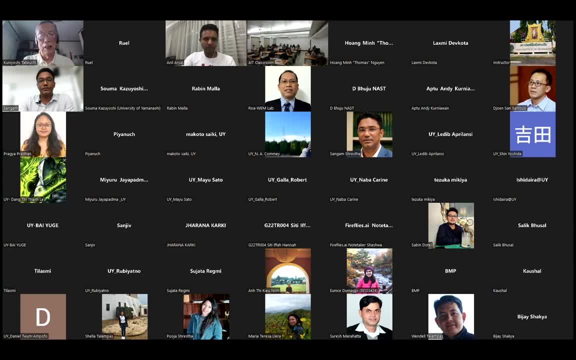 Well, no, they combine. You know, I said preparedness is very important to check the infrastructure or the you know warning. That is technical, Well, starting from observation, you know, but all those the technical thing or the infrastructure type of things, 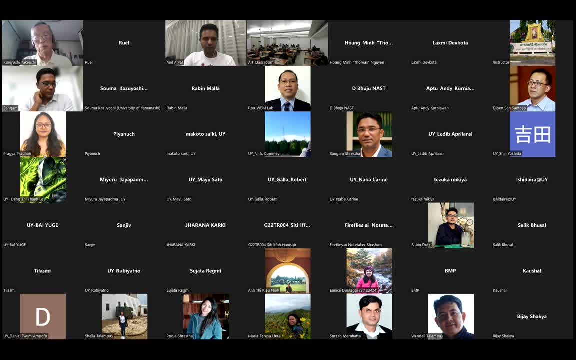 it's supported by people. People are using those infrastructure. So how to work those people- not only just awareness, but also working together- is most important for well, most important for preparedness, And that is why I said social capital. you know, social capital. 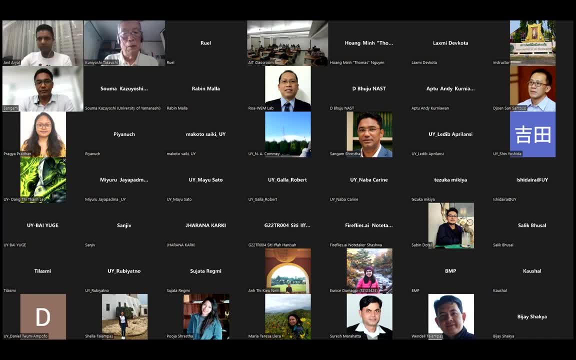 human relation is a power, And I said Sontoku is a saint of moral power. You know, moral is not just a discipline. This is a power to make development and economic efficiency possible. Without this, if we cannot trust each other, 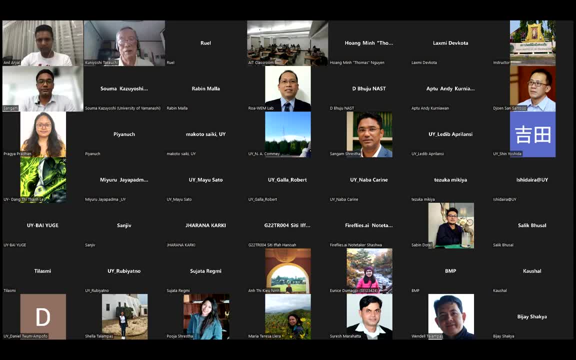 then we cannot do anything, See. So thank you very much for your question about disaster preparedness. Preparedness is not just technical or human awareness, but everything. So yeah, Yeah, thank you. Thank you, Professor Takeuchi. Are there any questions from the participants inside the classroom? 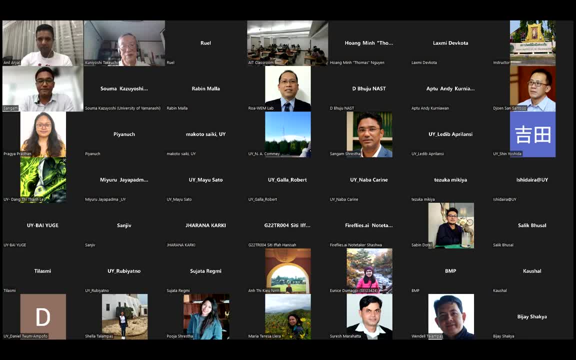 online participants. Sensei, can I ask one question? Okay, yeah, Dr Anil, please go ahead. Yeah, Sensei, one thing about: based on your so many years of experience in both academia and companies, what are your suggestions for co-implement actually? 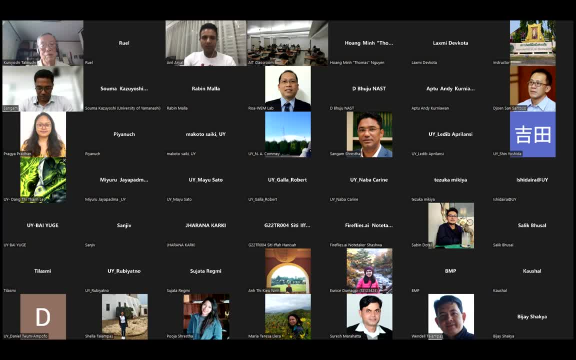 for the academicians, either restructuring the coursework or something like that, mainly in terms of co-implementation. Yeah, yeah, yeah, yeah. This is very, very difficult. the question too. Even you are student and you like to have paper published in science. 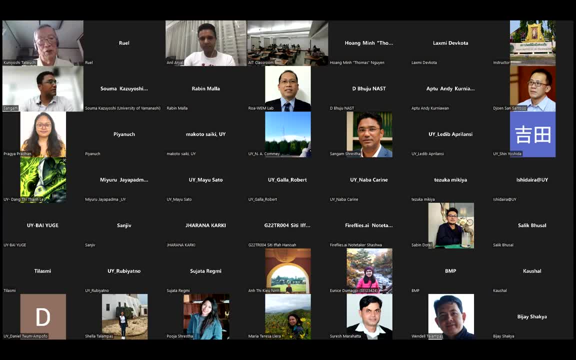 or you know good journal that makes your life possible. However, you should have a contact, or some contact, with real world And you have to do something, not just watching at what suggesting, but you do something Well in balance with your own. 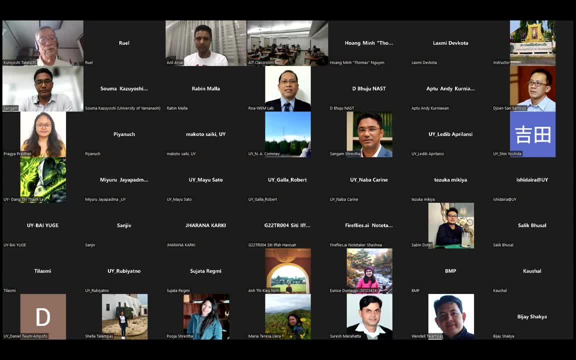 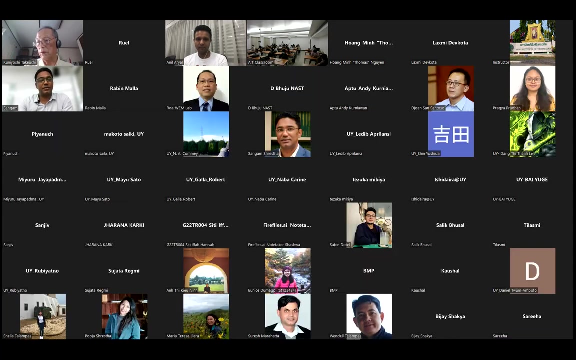 you know professional life. I think this it's very important in that transdisciplinary approach. it makes possible- And this is not just only your problem but also the professor's problem too. Professor has to, has to well accept. 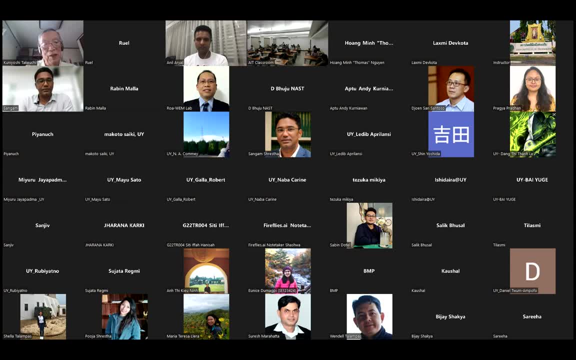 well, evaluate, value your activity in the implementation, And this should be in the journal too. Implementation or case study should be highly accepted in journal. So it is more like I'm saying this: we do need that sort of well. 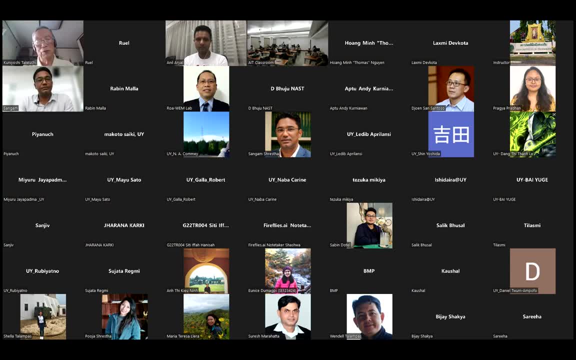 well, knowledge transfer? yeah well, some kind of infrastructure for this. well, I slipped away some keywords. Yeah, knowledge, we have to make sure the knowledge flow reaches from the source to the implementation place And the knowledge flow infrastructure. 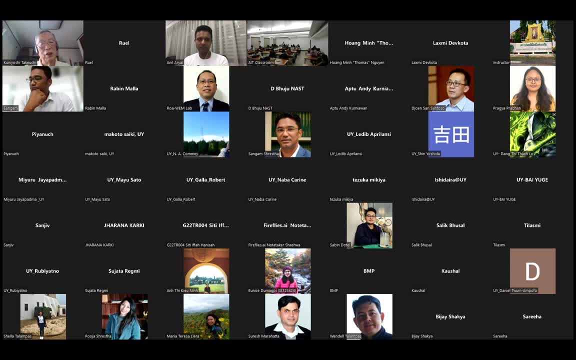 is necessary, And this infrastructure includes the publication or the assessment of the quality of your student activity as such. Well, thank you very much for your question. Yeah, Thank you very much. Nice to meet you. Yeah, Thank you very much. 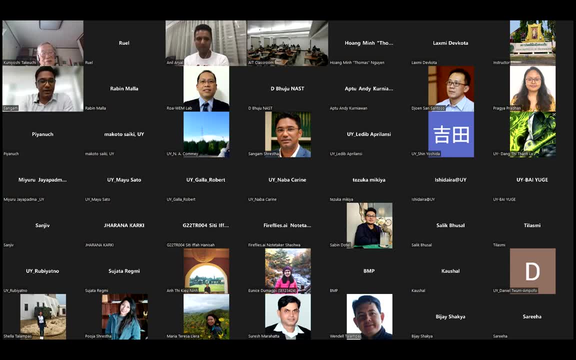 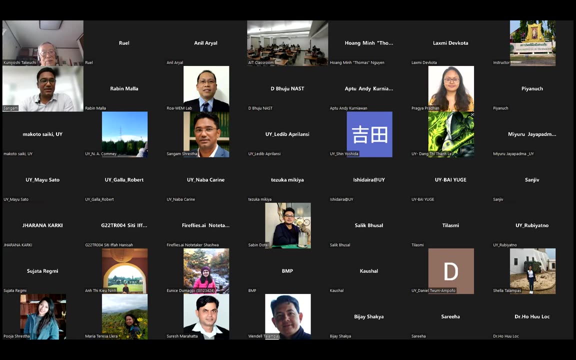 Professor Takeuchi. So are there any other questions? Any other questions from the classroom, inside the classroom, here? Okay, Sensei, maybe I have one question. Probably it's not polite to ask, but I'm just wondering, you know. 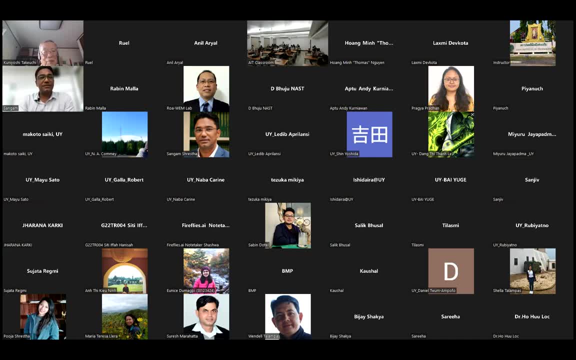 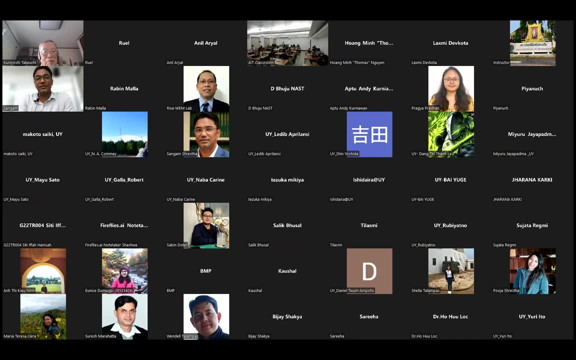 especially in developed countries. there are a lot of, you know, advancement in technologies, such as, you know, the rainfall forecasting, flood forecasting, and also a lot of the infrastructure in place to reduce the risk of flooding. But still many of the developed countries 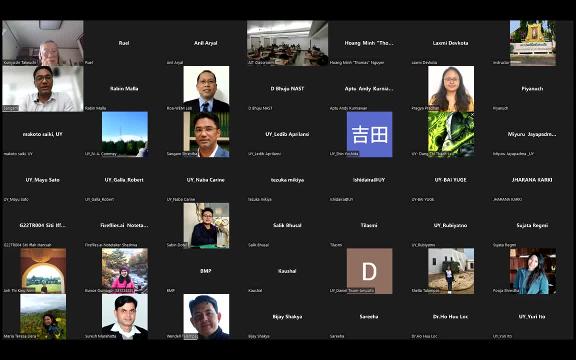 they are facing this flooding problem and also severe economic loss and damages. Okay, Can you tell what are the major reasons of, you know, failure of this flood risk management in developed countries? Well, Sangam, thank you for your question, But please think about the 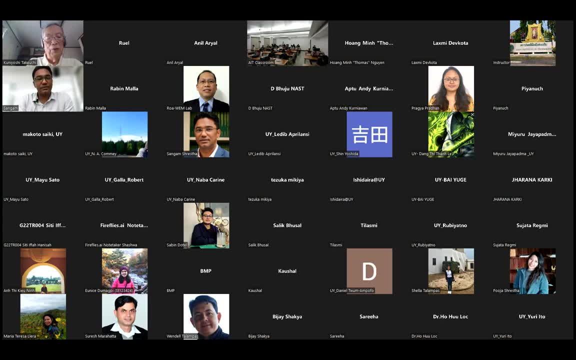 for instance, the number of people who die. It is declining and declining And sometimes, well, it reaches 200 or something. That's sort of 200 people died in 2018, or 2019 in Japan, If it happened 50 years ago. 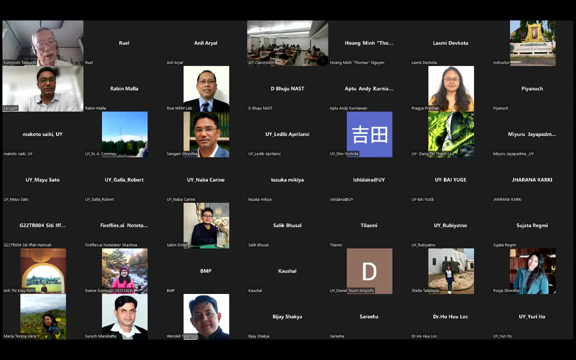 you know it should be thousands or tens of thousands of people. That is why you know the number of death toll can be reduced, But economic losses do not, And we have to face that. economic loss, Economic losses, doesn't change much. 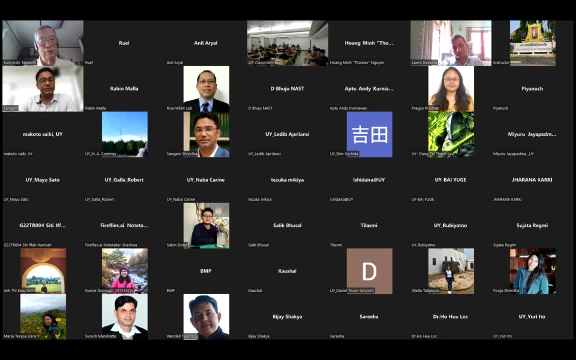 This is because vulnerability is increasing. Not we are failing, you know, in the management, But vulnerability increases. So even a small damage makes a very large impact. So the complexity of the society, including interdependencies or the value network, you know. 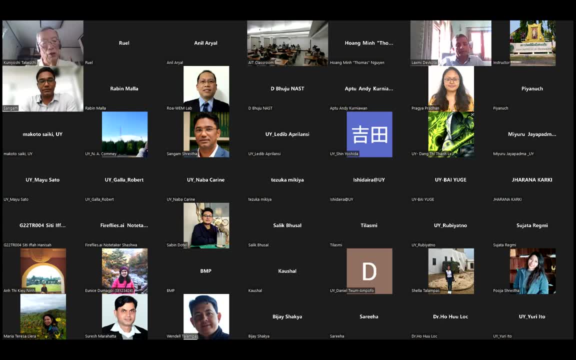 that makes the economic losses by disaster increasing and increasing. Yeah, thank you. Thank you, Professor Takeuchi. I think it's already two o'clock here, So it's time to close this seminar. And yeah, thank you very much, Professor Takeuchi. 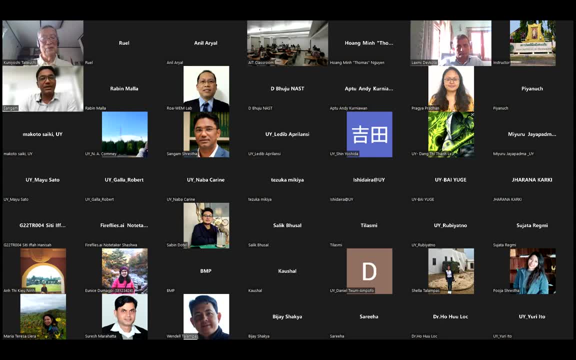 I think we're very fortunate to have this, you know, first seminar after your release of this book: Integrated Blood Risk Management. Yes, Yes, Once again congratulations, And this is very, very timely publication And I hope this will be very useful for. 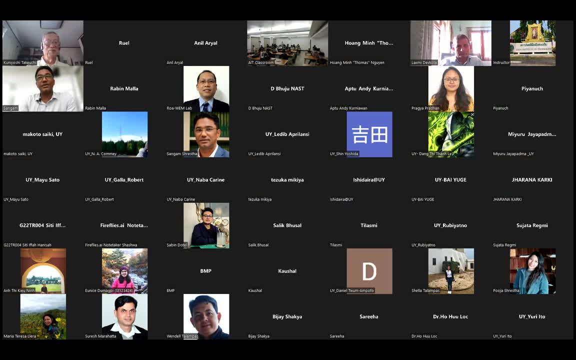 not only the policymaker, practitioners, but also for the students and academic institutions like us. Thank you very much, And I thank all the participants joining from several places And please stay safe and stay healthy. Thank you very much, Thank you very much. 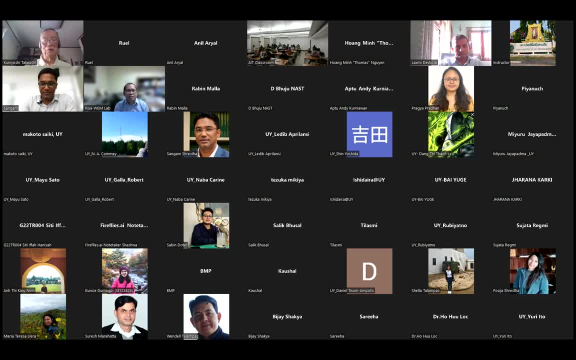 Thank you very much, Sangam. This was a very nice opportunity for me to express, explain the book And if well, if situation allows, maybe I'd like to visit once again AIT and the talk about this book, Yeah, sure. 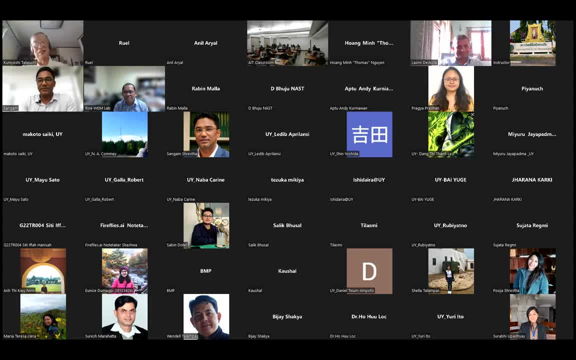 Sure, That is that maybe in some, in some cases. Well, thank you so much for your participation. Thank you very much. We look forward to meeting with you. Thank you, Okay, Thank you very much, everyone And those students attending this seminar. 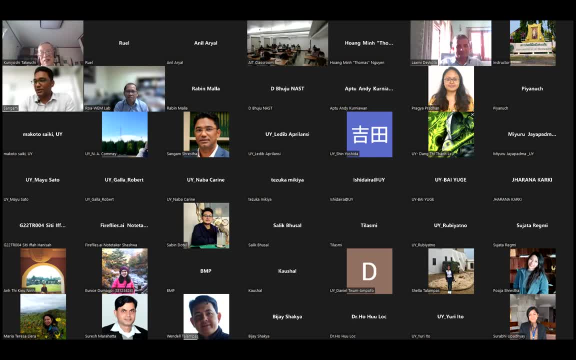 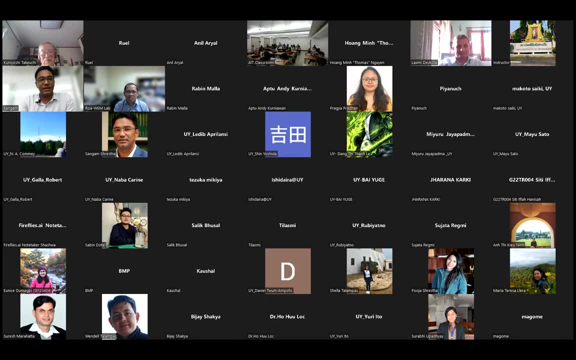 So I would like to request you to switch to another. you know usual Zoom meeting ID and password, So I will continue my lecture in another Zoom idea. Thank you very much. Thank you very much, Thank you.